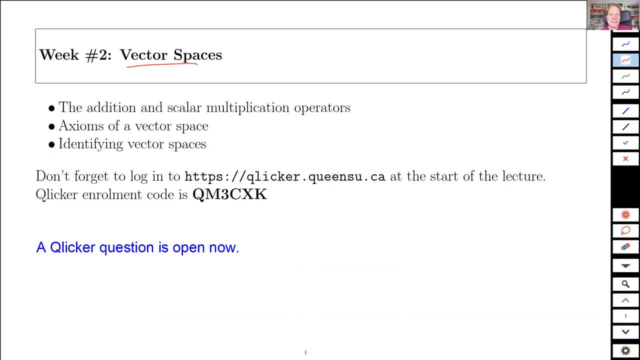 And as soon as we say that, bang, we have all these conclusions, all these results that we can draw on, And that's what we're going to be extracting this week out of the vector spaces- is just what kind of things can we immediately conclude if we recognize that? some basic rules. 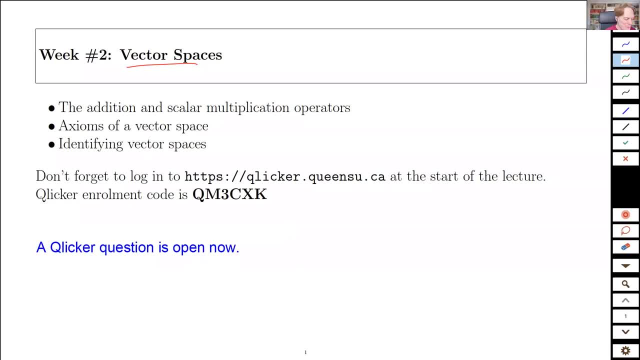 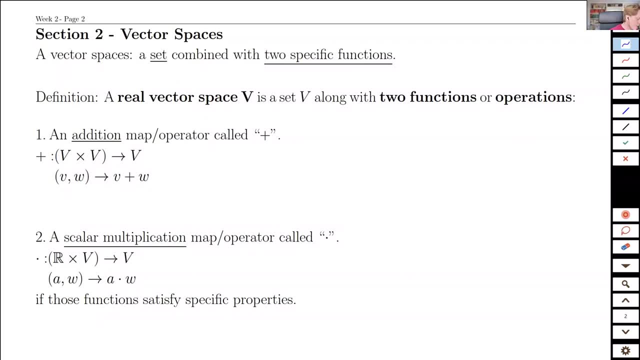 are in play with a set. So, with no further ado, let's dive into that. And what we're looking at when we talk about a vector space here is it's a set. So again, you just think of some blob of objects And what we're allowed to do. 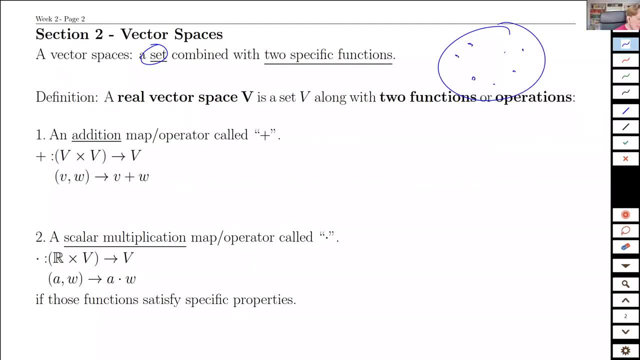 with that blob of objects. so imagine, a bunch of elements of the set is we can add an element to the set. So I can grab any two elements of the set and I can add them. And in terms of the function notation that we introduced last week, 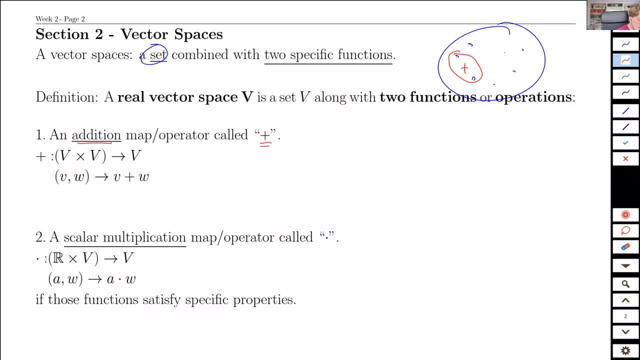 the addition that we're talking about takes two elements of the set we're working with. So we've got the set value and the set value, And so the addition takes two elements of v, two elements of v, and gives output a single element back. 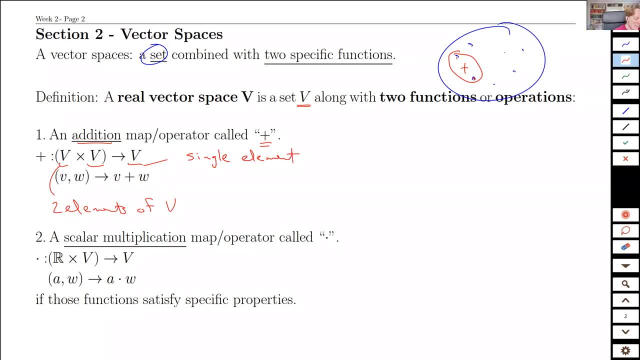 And again, this can either feel very abstract or just obvious, because if you think of adding two real numbers, you get a real number back. Okay, that's fine. And remember, this cross thing here is the Cartesian product. So this is the name of our function. 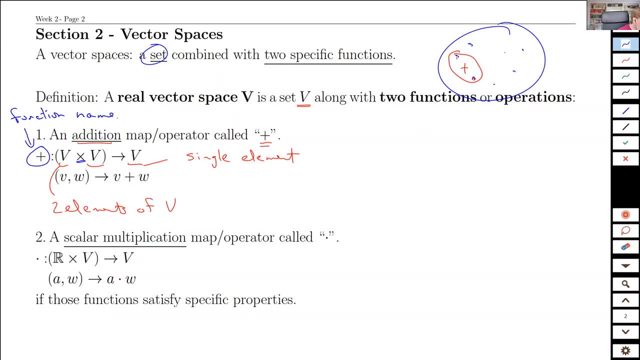 our function name. This x represents the Cartesian products. We're saying I have a pair of inputs, both of them elements of v, and then I get an output that is the sum of those two things. The other thing we're going to throw on is the real line on the side. So the real line is going. 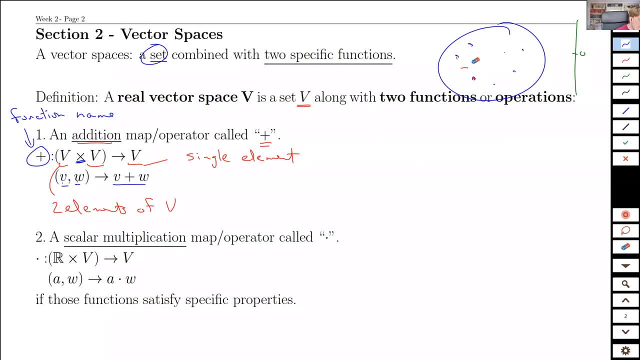 to be something that comes into play with these numbers as well. So we might decide to take one element of our set and multiply it. We're going to use the dot product looking thing, the scalar multiplication, say with a number like minus two, So we're going to be able to combine real 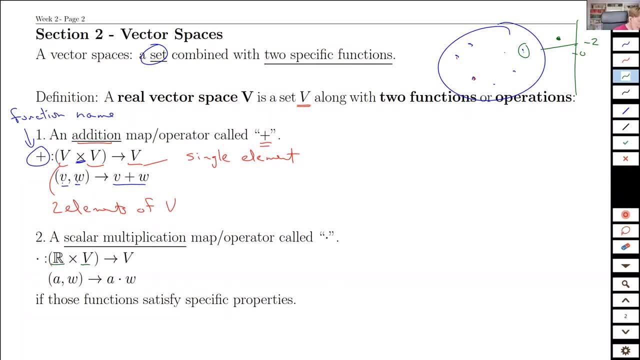 numbers and these elements in the sets. We see that in the notation here as a real number and the set that we're working with. So we combine two of those and we get a new element of the set. All right, let's make this a little more concrete. 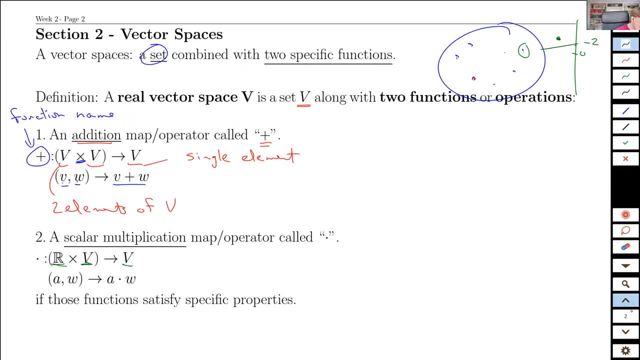 Or sorry, a little bit about nomenclature. first, This is called this combination of a set vector along with the addition and the scalar multiplication is called a real vector space, And the real part there comes from the thing we're allowed to multiply by in our scalar. 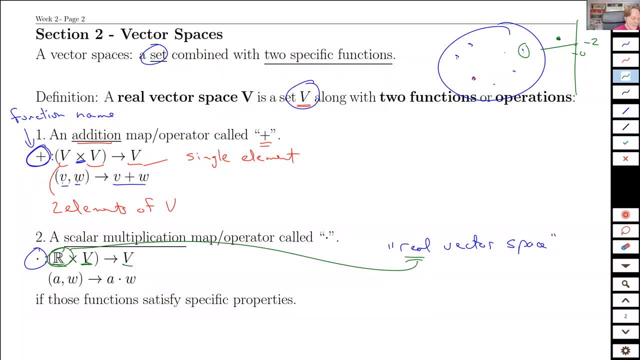 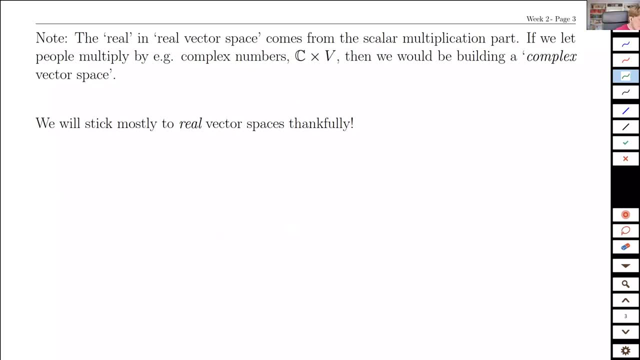 multiplication being real numbers only. Now, for those who are going on to Apple Math and Fizz, you would not be surprised to hear that actually even ECE, especially the electrical side, is going to be able to multiply real numbers by a set number. So we're going to be able to multiply. 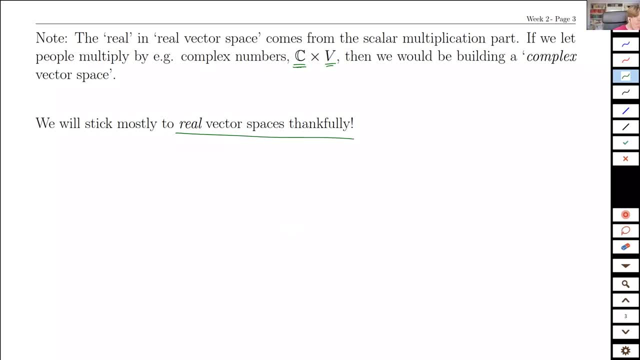 real numbers only by a set number, by the number we're going to be multiplying by a set number. And you can see, here we're going to multiply real numbers by a set number, And so what you'll see is that in this class there is the possibility of taking complex numbers. 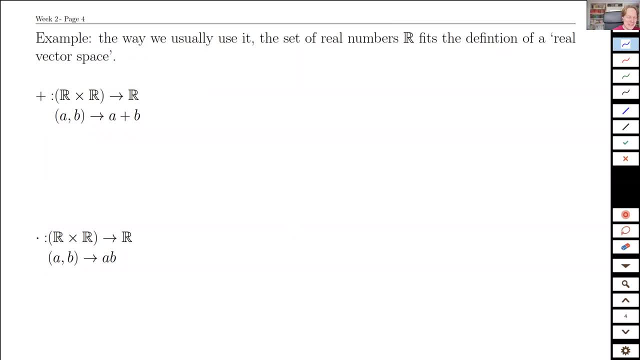 times our set numbers. If you want to do that too, we are going to stick in this class pretty much to real vector spaces, So kind of thing you're more familiar with. So here we have our set V, which is the reals now. 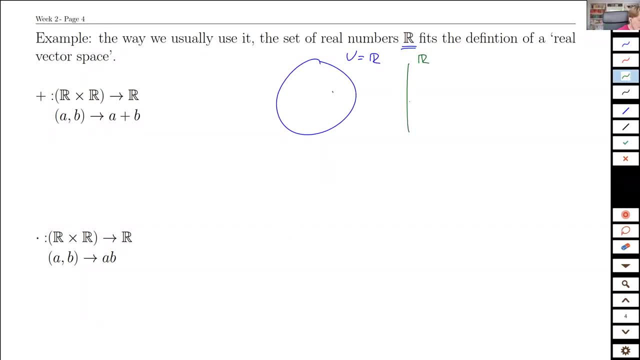 and we also have the real numbers that we can multiply by. It just happens to be the same set. That's fine. So when we take two real numbers we can add them. So we would imagine taking three plus four. Well, in this notation here we'd say: 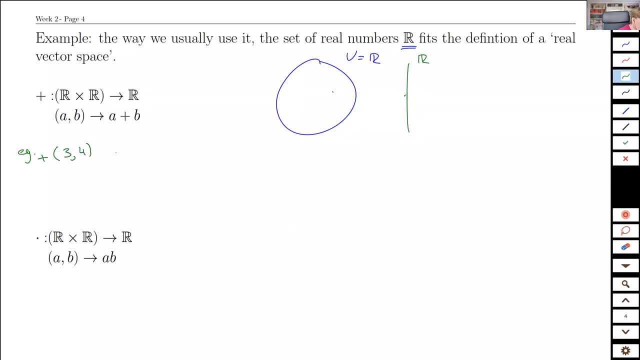 I'm gonna apply the plus operator to three, four. That's gonna turn into three plus four, And typically when we get to this stage in the calculations we go: what rules are we using for these kinds of calculations? Well, now we're just down. 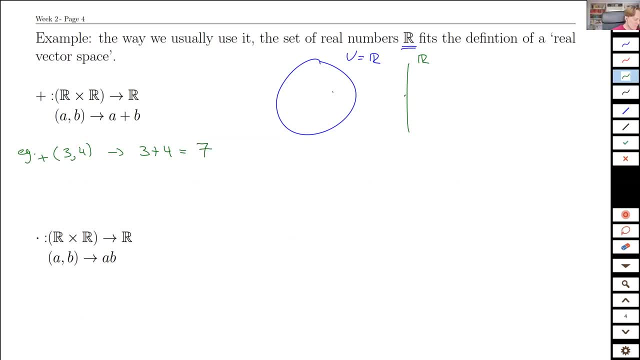 to regular real number operations, and so we would get seven. But you can see that the plus operator takes in two elements of the set we're working with and gives another single value back. three plus four, Two real numbers, gives us one single real number back. 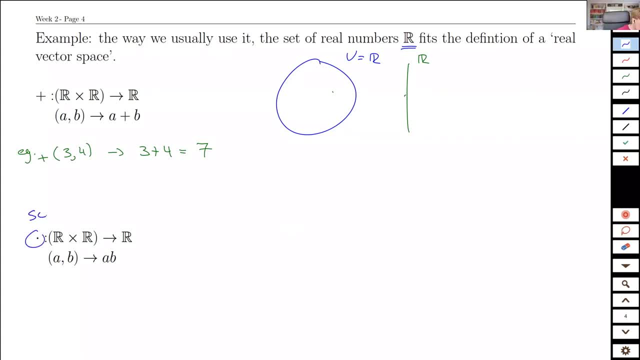 The dot operator, the scalar multiplier- again just reminding you what that means- is the scalar multiplier? It has the same rule, except now one of the real numbers comes from the set. So I grab a real number from the set. 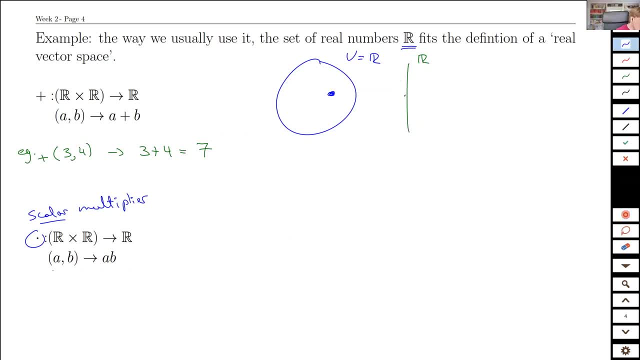 and then I multiply it by another real number as a scalar multiplier. We can't really see that in the math, but it's helpful to think about it that way when we get to other examples. So here, yeah, if we take the dot of two and seven, 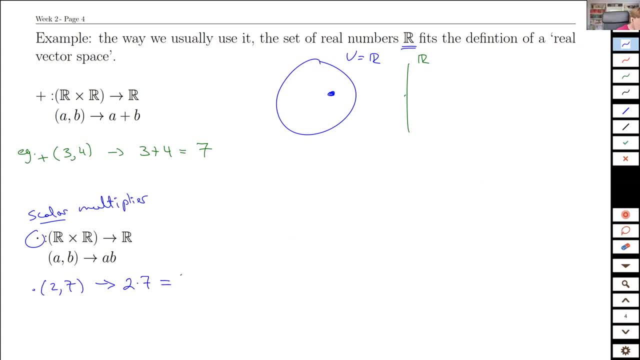 we would get two times seven In regular real number terms, we get 14.. So again we get, okay, get. If we input two real numbers, we're going to get the product of them, like we'd expect, And so this is what you do every day with real numbers. anyway, We're just giving a little bit. 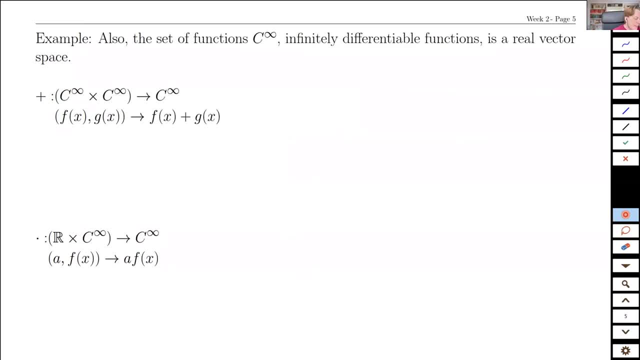 of a framework. It's not the only vector space that you've seen, though. A more interesting set is the functions. So it's a set. Our set of functions now is C infinity. This is the continuous and infinitely differentiable functions is also a real vector space. 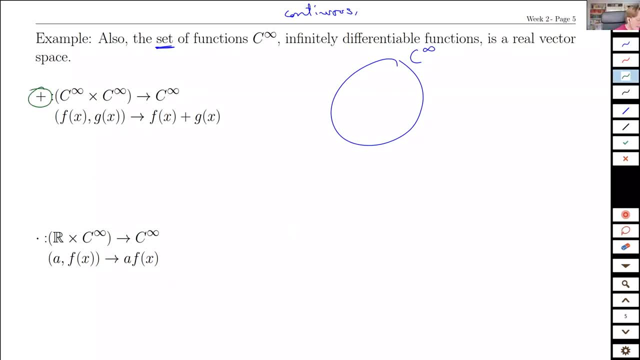 Now, what do we mean by that? Well, it means that we can add two functions. Okay, All right, But I think most of us feel a little shakier about that, because it's something we don't have as much experience with- but you've done it before- And specifically what we end up. 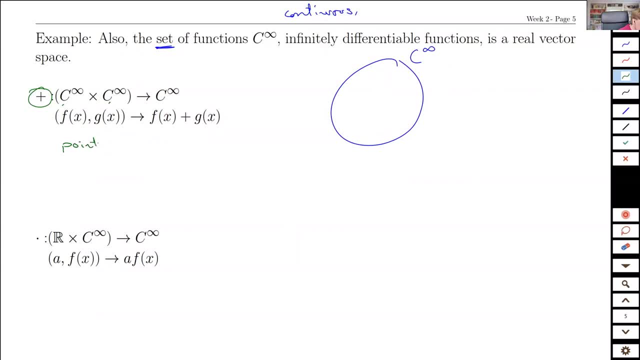 defining is point by point, Point by point sum. So if we have two functions, F and G, we can add them together and we get the new total, which is at any point X. I'm going to find out what F gives me at that point I'm. 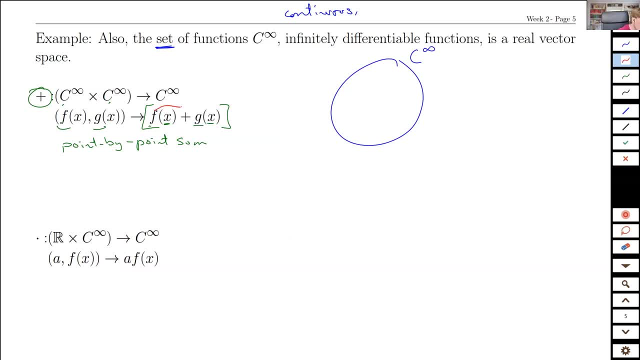 going to find out what G gives me at that point And I'm going to use regular- Now we're at this point here- regular real number addition. So we define the addition of functions By point, by point sums, And then, when I get at each point, I'm just going to use regular. 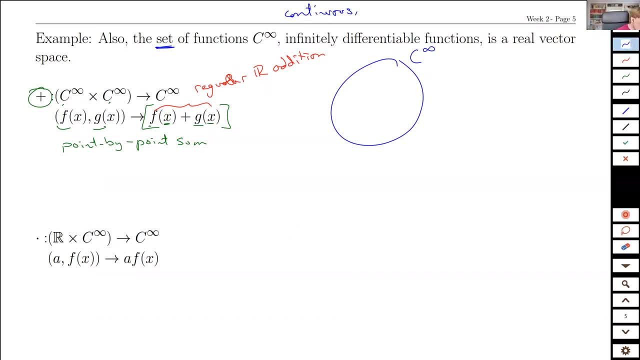 real number addition. We're also going to have the scalar multiplier here, And now we see kind of that contrast between the two inputs. that's possible. So if I have a real number and I multiply it by- sorry, I'll show you an example here. My apologies, Let's do an example. 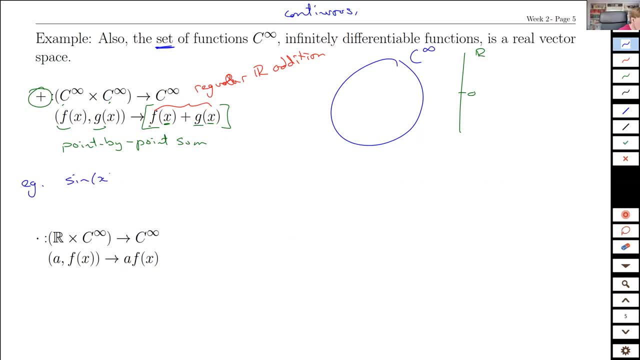 of say it's going to feel just vacuous, but sine plus- Actually- here's how we usually write it- Sine plus cos of X. How do we actually compute that? We actually compute it as sine of X, get that? 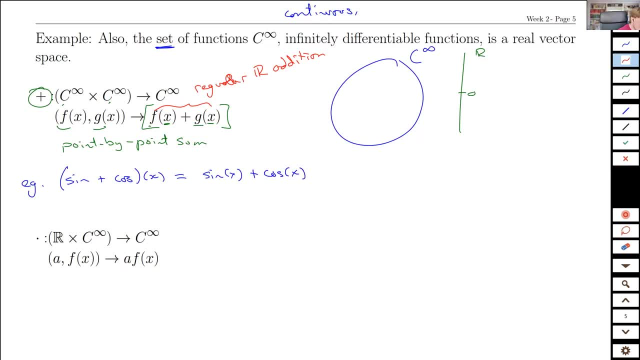 real number and then cos of X. So this is kind of without the X value. This is what we think of as our function. It's just the operator, the transformer, And again this is gets a bit into the weeds about the notation. We don't tend to get too fussy about this. It's just as long as 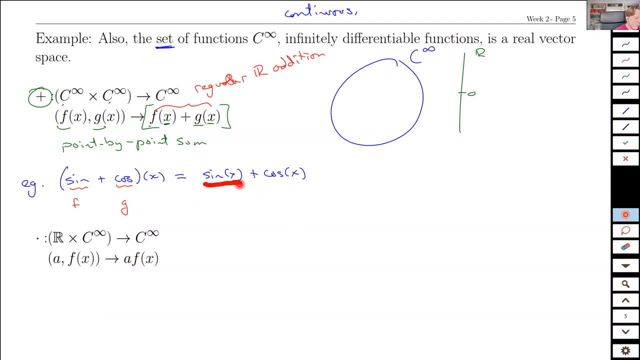 we? someone says: oh, I'm at the sine function, the cos function, I want to add them. What are you actually doing? You're adding both functions together, point by point. Someone gives you an X and you can figure out the sum by transforming each one of them and then adding that. 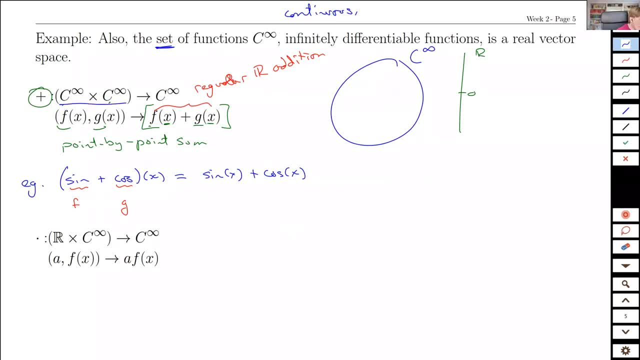 Yeah, the multiplication symbol is separate. So this is about the set, This is the input set or the domain, And so that cross in there is just saying that it's the remember Cartesian multiplier or Cartesian set multiplier from last week. So I have one set and another set. 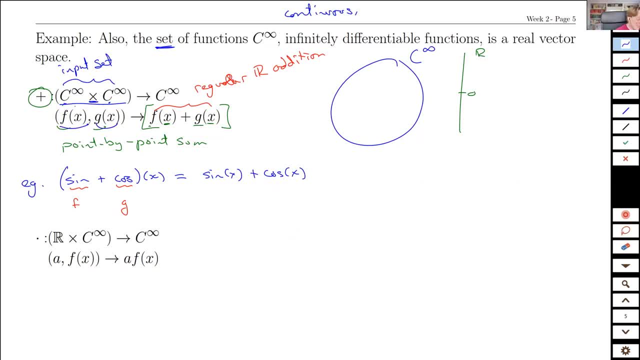 It basically means I'm going to get a pair of elements that are going to go into the input here, So I can't add one function. I need to add one function to another. I need to add two functions together, And likewise here I can't multiply a function. I need to multiply a function by. 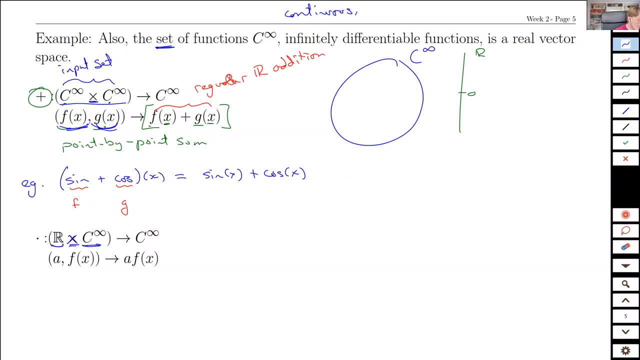 something. So this Cartesian product here is saying: when I do multiplication, scalar multiplication, I need a real number, And then I also need a function, And then I can combine those two things to get a new function. And in fact this is the same as up there. It's a point by point. scalar multiplier. 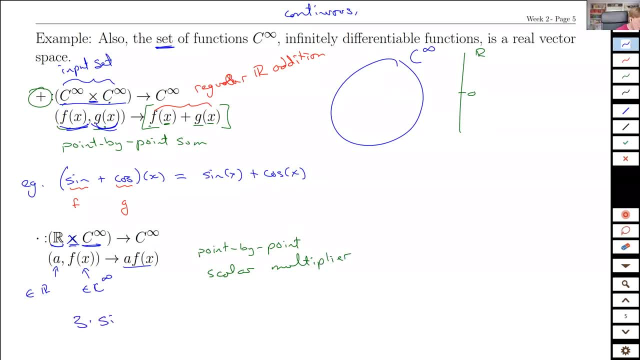 So what do we mean when we take three times the sine function of X? Well, what we mean is we're going to take sine of X and we're going to multiply it by three times the sine function of X, And then we're going to multiply each of those numbers by three with the regular. 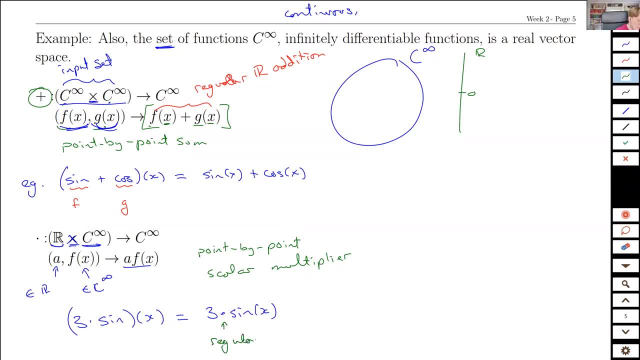 real number multiplier. So again, this can feel very abstract, and that's fine, as long as what we're trying to do here is identify and explicitly identify that we're doing these kinds of things with functions, this idea of a scalar multiplier and addition, And the rules are the same as 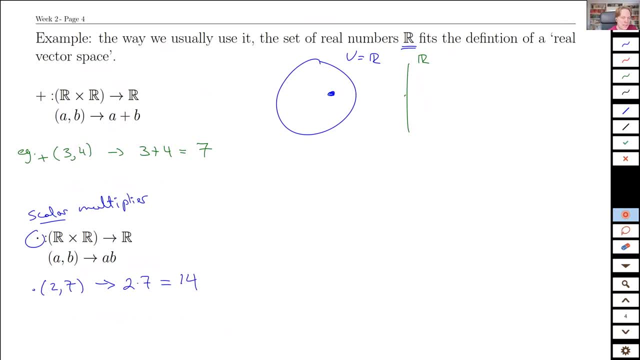 well, we're going to do this, when we do this, when we do that kind of thing for real numbers, And what we're going to see is: oh okay, if that's the case, then maybe there's some other rules, some other undefined things that we can tease out of that And then also tease 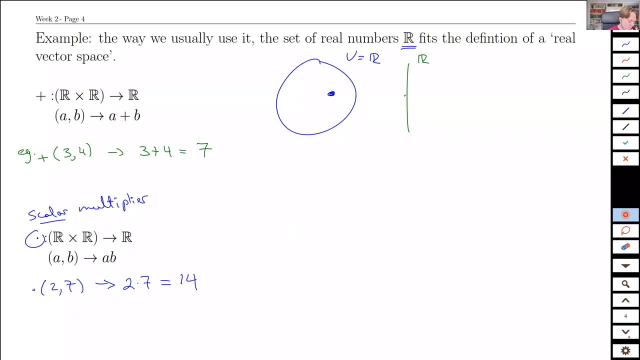 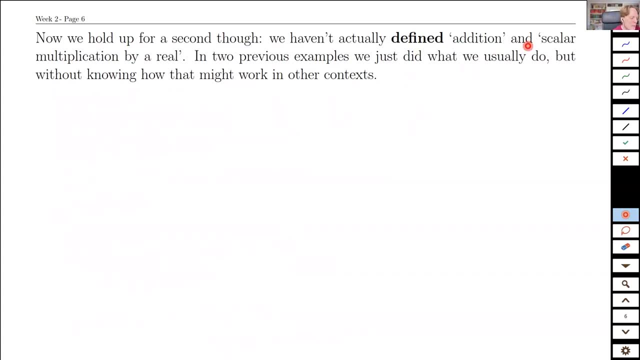 out some consequences that might apply to new sets that we haven't thought of. So these ones are reasonably familiar. The thing that gets us into grief right now is: you know what do you mean by adding and scalar multiplication by a real? Are the rules to that that we haven't really touched on? And there absolutely are, In fact. that's what our next lecture is going to be about. We're going to talk a little bit more about that. And then we're going to talk a little bit more about that. And then we're going to talk a little bit more about that. 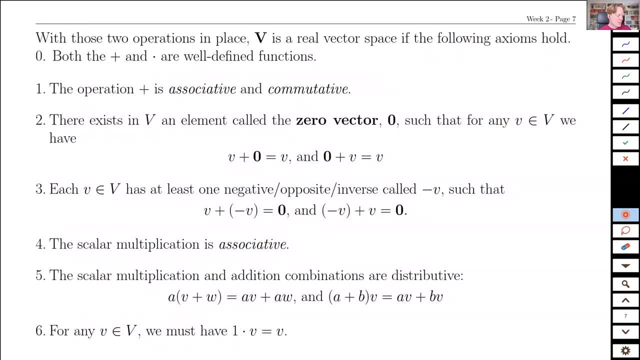 The next page here is: this is sort of a summarized version of- I think it's- eight forms of the axioms of a real vector space. Sorry, I should put a highlight on here. These are the axioms of a real vector space. And what does that mean? Well, axioms are: 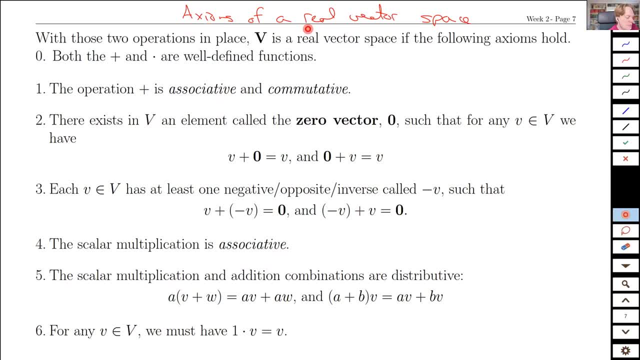 fundamental beliefs about a system. So if we say we have a real vector space, then we say that each of these things that we're putting in here is true. That is what we believe is true. Also, if you can show that these things describe a particular set and an addition and scalar. 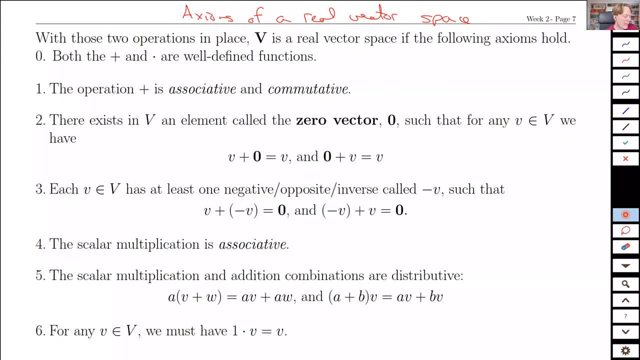 multiplication, then you have a real vector space. So there's this little duality between those two. but axioms are sort of fundamental beliefs, All right. So there's an important zero thing here that comes into play, which is that the plus and dot scalar multipliers are well-defined functions. 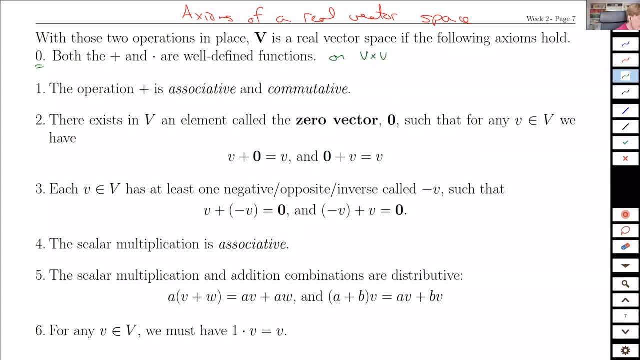 on v cross v and the real numbers cross v. What does that mean? It means that the function is defined And actually- let's make it more explicit here- Plus and dot are defined for all inputs. In other words, there's no domain issues. So I can put any two numbers, any two elements of my 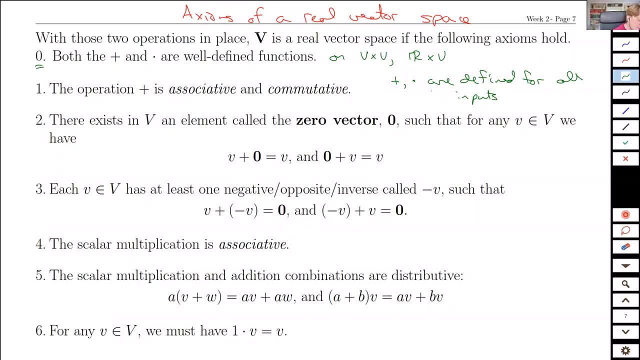 set together and add them. I can put any two numbers, any two elements of my set, together and add them. I can put any two numbers, any two elements of my set, together and add them And still get something back. And also any real number times one of my set and get it back. 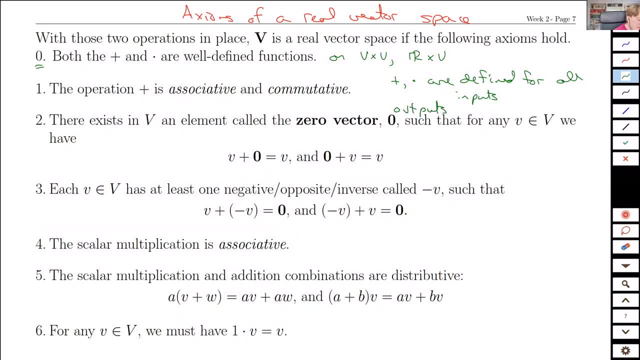 And the outputs are all in v as well. So I remember each of these things. if I add two elements of my set, I'm getting another set. back to green, I get another element of v. When I took a scalar multiple, I also got another element in my set. 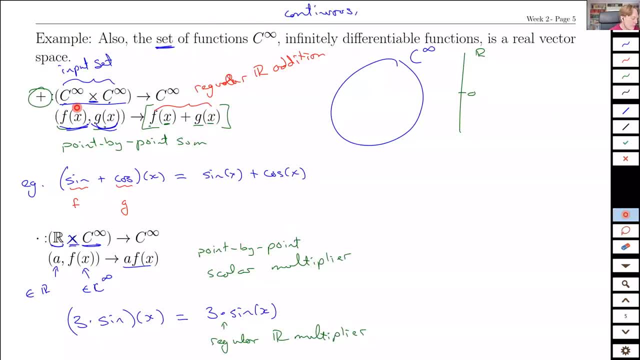 Going back a slide here for a second. When I took two functions and I added them together, I got one new function back. That has to be defined for every possible function. I can imagine- And we kind of take it for granted That's true- that 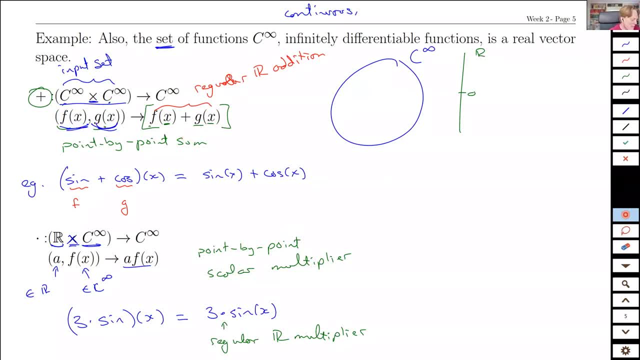 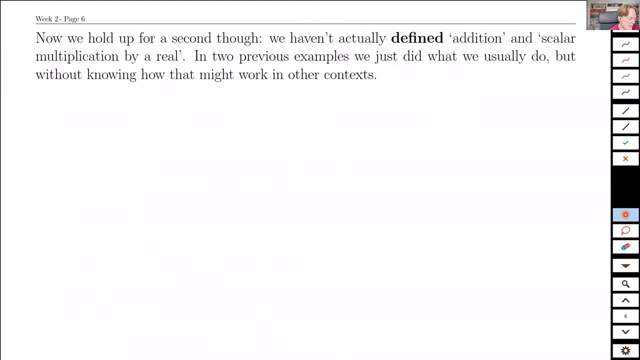 we can do this, but it's actually a little more subtle than that, So we have to investigate that a bit. Also, if I scale or multiply any function, yeah, I'll get a function back that's still in my set. So that's often a big tripping point, as we'll see when we take a look at some. 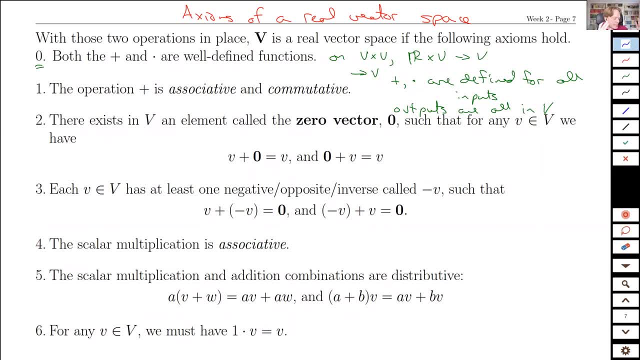 examples of things that are not. But let's take a step back and go all right. what else is in this set? And it's again, it's this weird feeling of stuff that you know but maybe haven't formalized before in your mind. So the rules of this plus operator is that it. 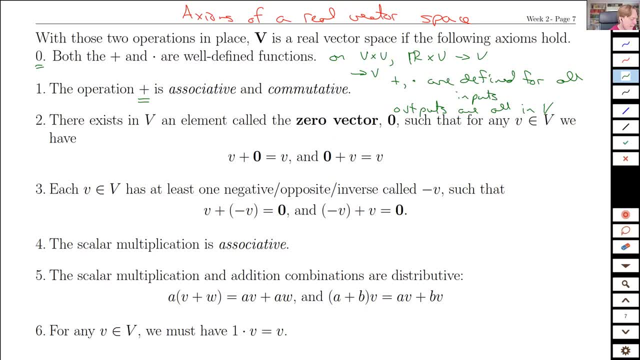 has to be associative and commutative. We'll talk about that in a second. There has to be a zero vector, or zero element, sometimes called the zero element. Well, what do we mean by what defines a zero element? Well, it means when I add it to any element, the element doesn't change. So we're like: 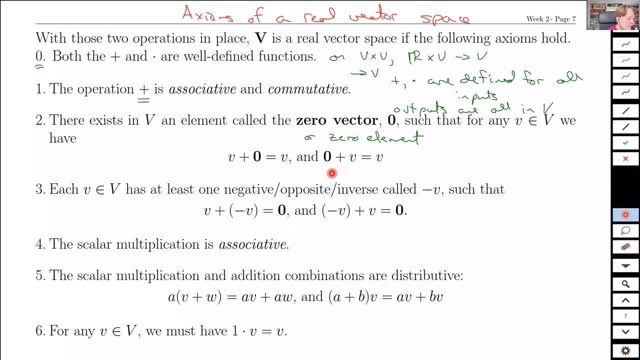 oh, what does zero mean to me In terms of vector spaces, the real numbers. if I take a real number and I add the zero real number to it, then I get no change in my number And order doesn't matter. That kind of goes with the commutative side here. So having that in play actually turns out to be. 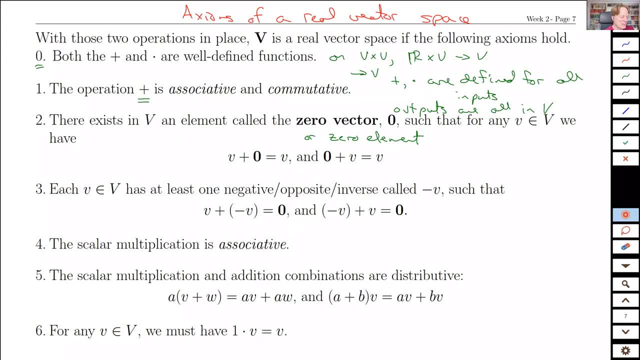 one of the fundamental building blocks. You can't do the math we want to do if that's not the case. There's also this idea of, if you like, additive, reciprocal. There's two things that I can add together and get the zero vector back. So there has to be a zero And for any set element there, 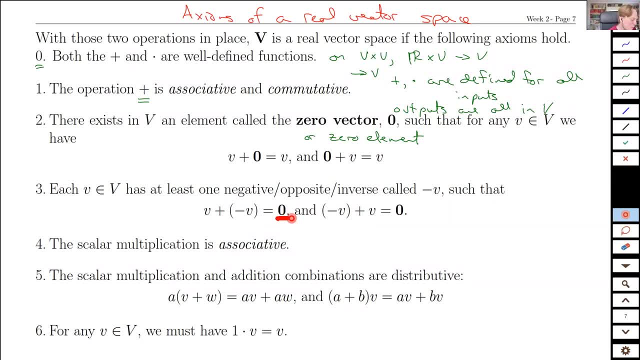 also has to be something that takes me back and reverses that and gets me to zero Again. associative things for multiplication. So these are all about addition And then we get into the multiplication and combinations of it. Scalar multiplication and addition are distributive. 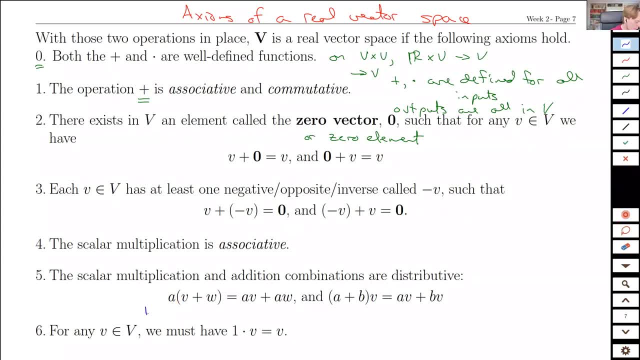 So if I take a scalar multiplier here, so this is my real number times two elements of v- I guess it's already in there. I'll put an element in v. Oh, that's horrible. So this is an element of the reals, And then I take my two elements here. If you take a 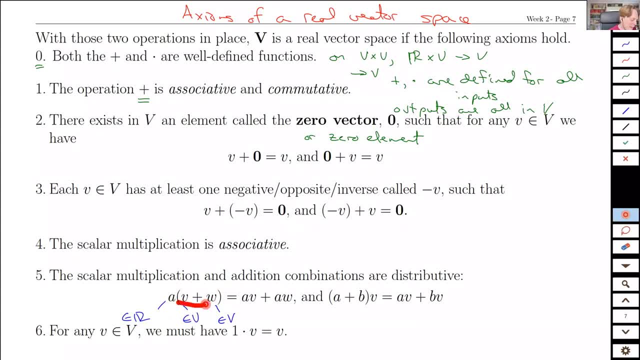 careful. look at what's happening here. we're doing a scalar multiple, after I do addition, versus scalar multiplication, and then addition second, And those have to give us the same amount. So again, basically, the rules that you already know, but we're just saying it turns out this is a fundamental rule- that we can make this kind of association and get the same value back. 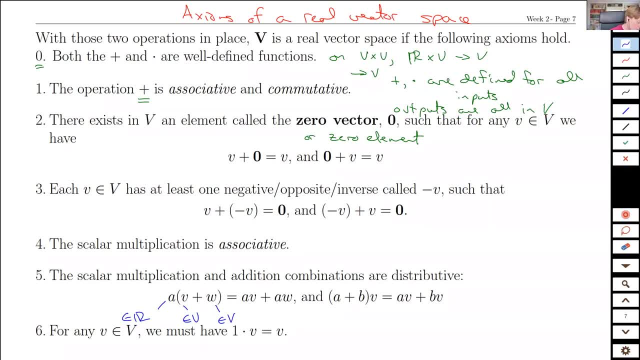 And there also has to be a unit multiplier. If we multiply things by the number one in our set, by our real number one, we get the same number back And again, this is like obvious. What else could you get? We will show you examples where you can get something different if you play around with what addition and scalar multiplication mean. 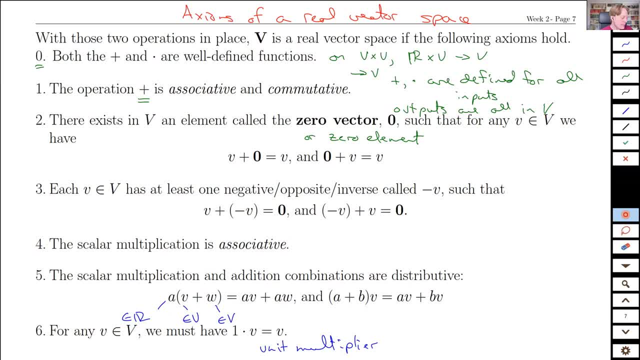 All right. So axioms are real vector space. This entire block here. These were never sorry. what are we going to ask of you for this? You should know these loosely. We are never going to ask you to produce a list of all of them altogether. 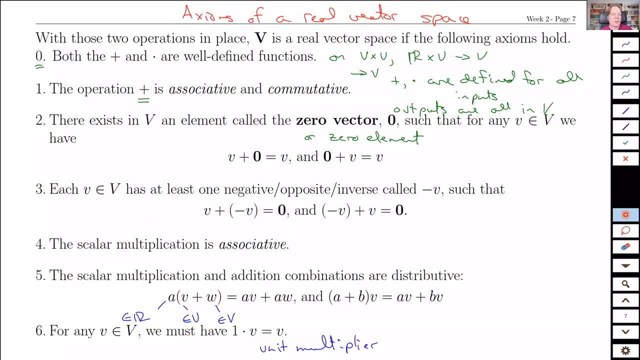 That's not going to happen, But you should recognize them and know that they're in there And with a prompt like: show this Show that there is a zero vector in this set or in this vector space. That is the kind of question we do. 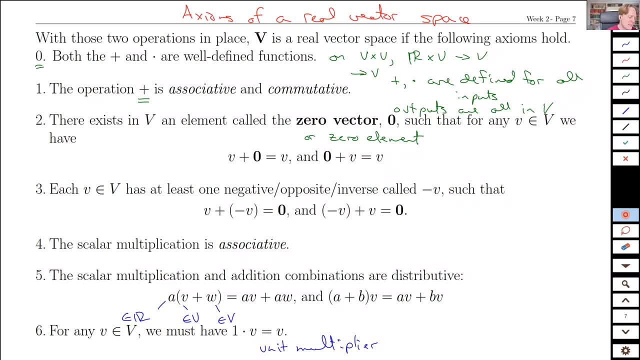 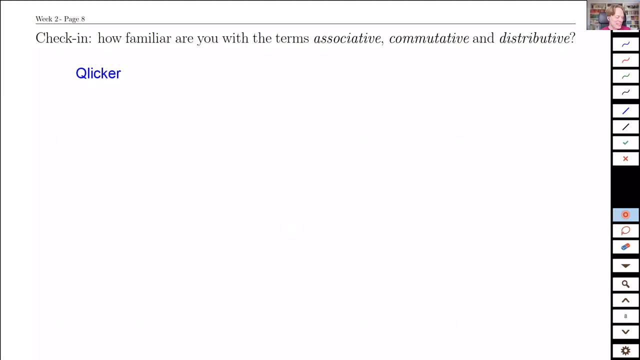 So we remind you of one of the axioms and then ask you to do something with it, And we'll see examples of that as we go through this week. All right, Part of this hinges on your own understanding of terms like associative, commutative and distributive. 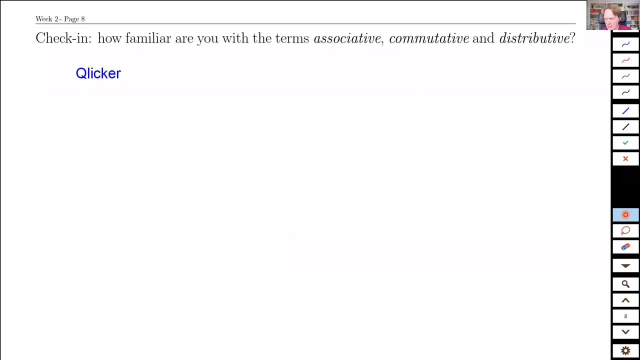 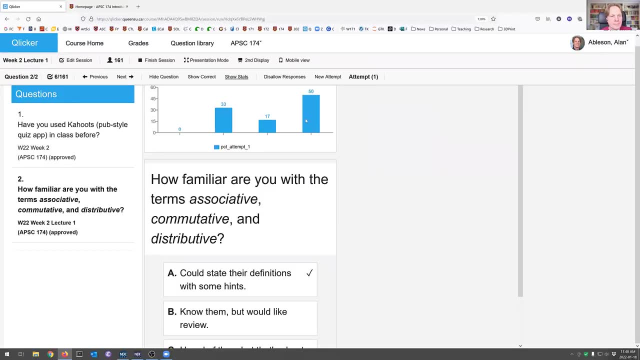 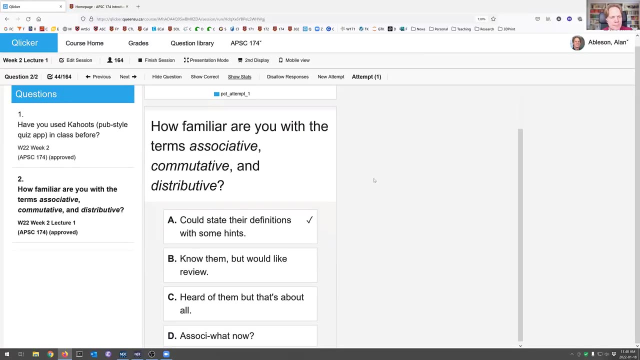 So just for my own benefit here, I just want to check in and see what those terms mean to you. So click over here. Actually, yeah, bring it up. And again, all these notes are online in the APS-C 174 on Q site in the lecture note page. 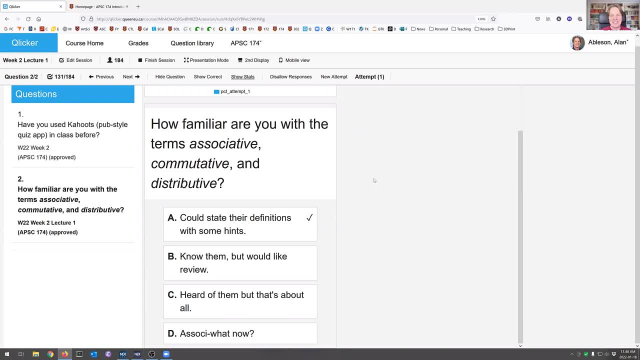 Okay And Yeah, all these things are kind of vacuous until we get some context, some examples. So that's what we're going to work through over. the next little bit is: what does it mean? What do you mean by the additive inverse? 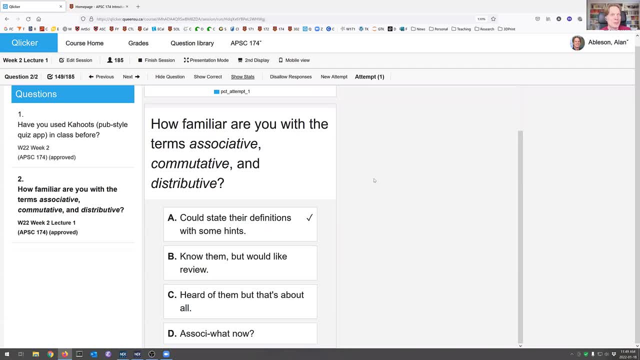 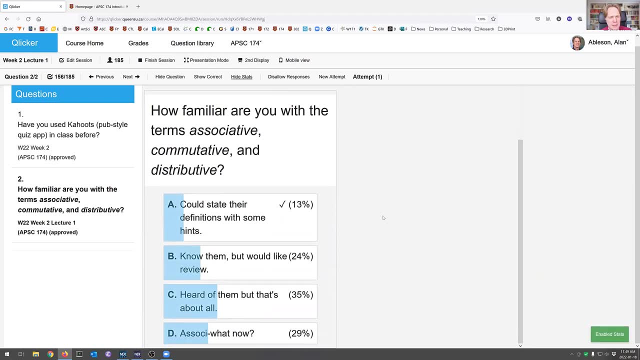 And what do you mean by the zero vector And what does that mean in different and some of them, some new vector spaces as well as the familiar ones. So all right, And we do for that. Sure Stats for them as well. 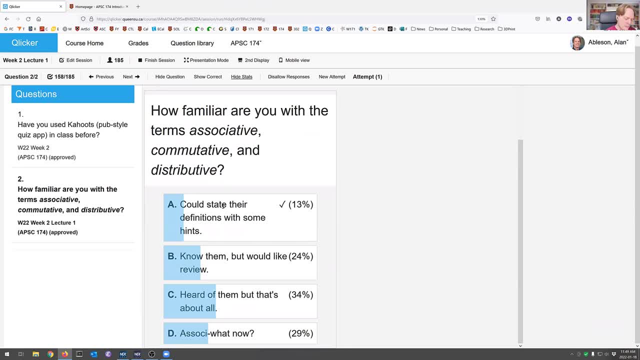 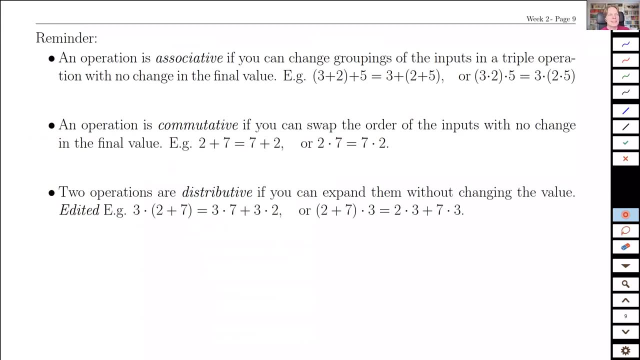 Okay, Okay, All right, So I'll spend a little more time on these next couple of slides here. Let's go back to here. So again, we're not going to ask you to say what the definition. yeah, I don't think we've ever asked students what the definition of associative is. 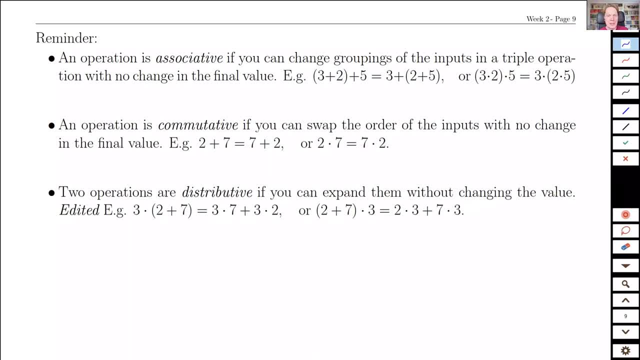 It's things that you do already anyway, though, So it's kind of nice to have a name for these rules that you might have applied. So association is grouping right. People associate together, they're grouped together. So an operation like addition is associative. if I can associate these ones first, 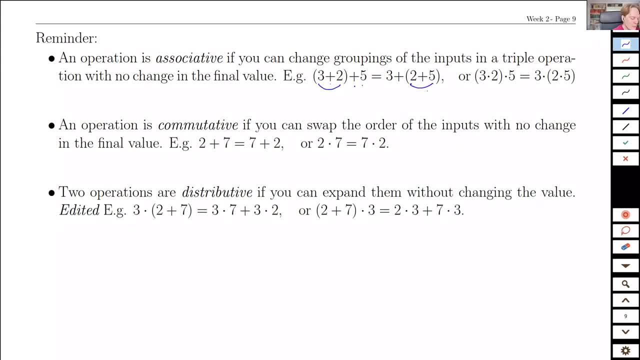 And then add the second one, or if I can associate these two first and then add the first one. So essentially it's order doesn't matter, but not in the commutative sense. The sequence in which I do these or group these terms doesn't matter. 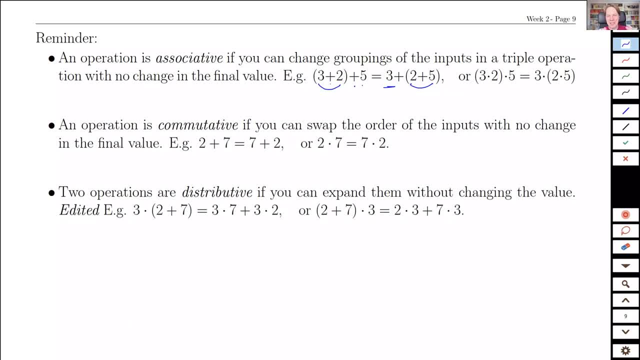 This gets you into whole order of operation stuff, that kind of stuff, And for our purposes it's important to recognize that it's true for both multiplication and scale. sorry, addition and scalar multiplication there, Commutative, All right, Okay. 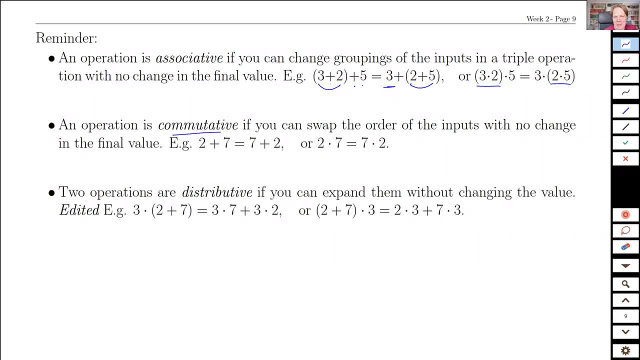 Commutative- I haven't got a good analogy for this- like commuting back and forth, I don't know, but basically swapping the order. If you change the order of these operations, or, sorry, order of the elements in the set to first, then seven added to it, or seven first and then two added to that, it doesn't matter. 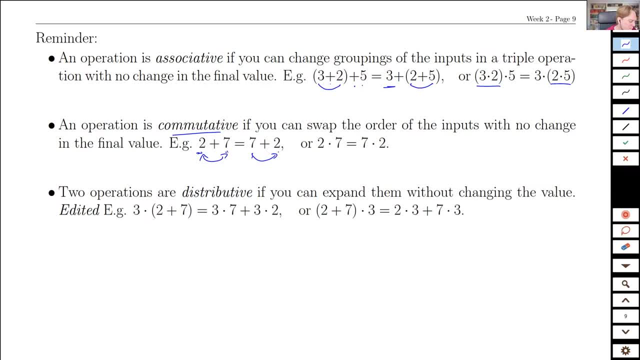 That's going to be true for all the rules we're working with as well- And distributive is when you combine the two things and you have a scalar multiplier outside, scalar multiplier outside, And then you have the addition inside. And just recognizing, you do this all the time with polynomials especially- hey, I've got this multiplier out front. I'm going to multiply into all the terms inside. 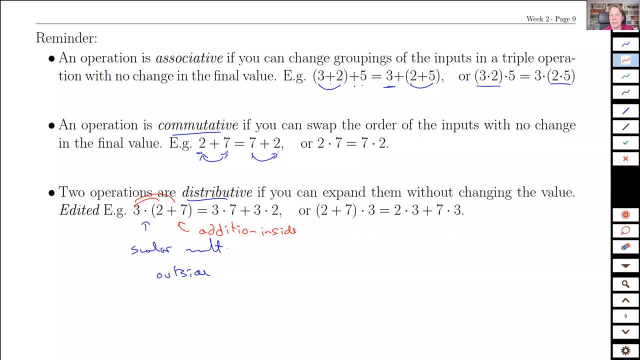 That's what the distributive property is. It says you can do that, You don't have to think about it, It's safe to do that. The result you get is equal to what you would have had if you had Started or left it in its original form. you get two things that are the same quantity, and it works whether the multiplication is sort of first- sorry, the summation is first and then you multiply, or whether you multiply from the left. 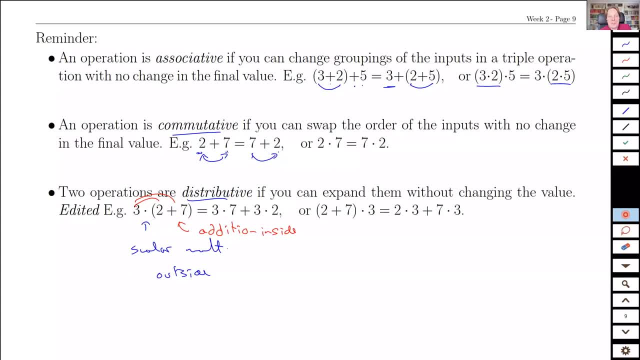 And again this all feels like what else could it be You? we will see actually cases where this distributive feature actually more like commutative. commutative is not going to be true for matrices or many matrices. So If anyone's seen matrices before, represented by large numbers, sort of a grid of large numbers. 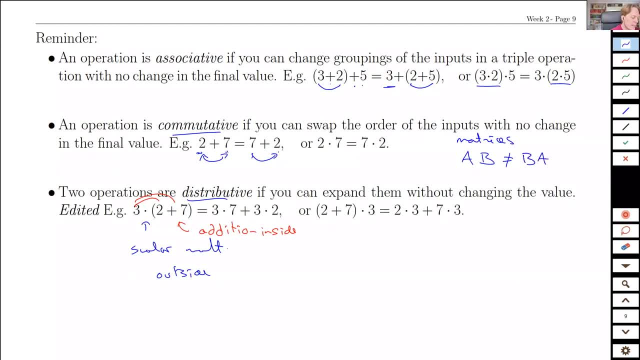 With matrices. it's not true in general that I can swap the order, even though it's still multiplication. It's not this kind of multiplication that we're talking about here. So matrices Multiplication is not commutative, So it is possible to come up with things that we're interested in which do not. 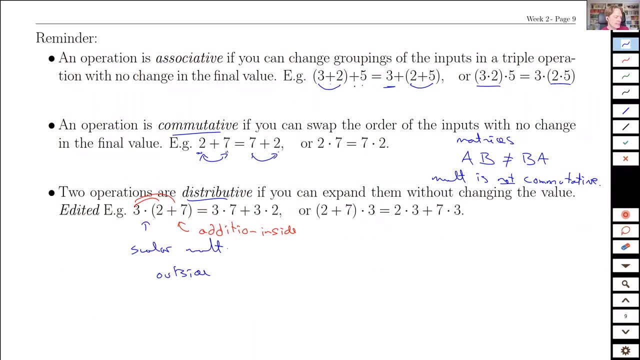 Satisfy these properties. All right, So that's just a quick thing. So associative is: I can put brackets around things and not change the values commuting, as I can change the order, actually the numbers, in my operations and still not change things. 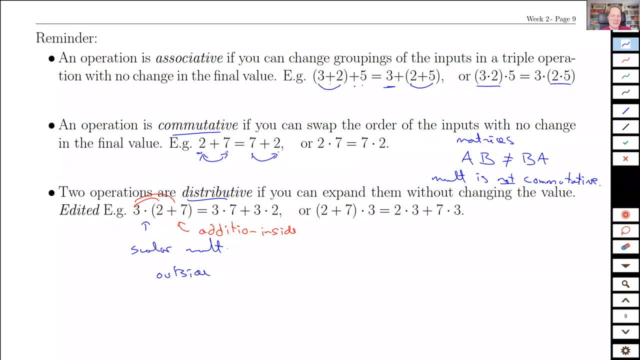 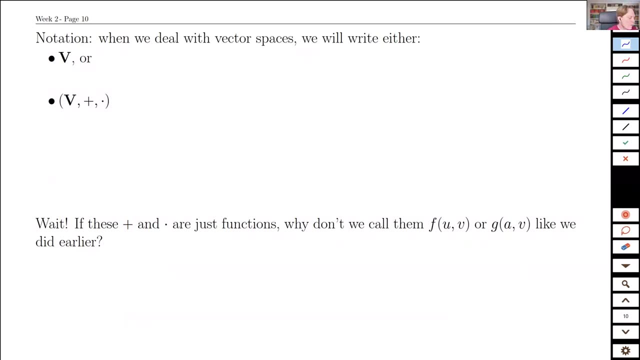 And distributive is the multiplication outside can be turned into multiplications inside, added together at the end. all of those, without changing the value of what we're trying to calculate, All right, All right, All right. So notation: If we have vector spaces, we can often just talk about the vector space that we mean. 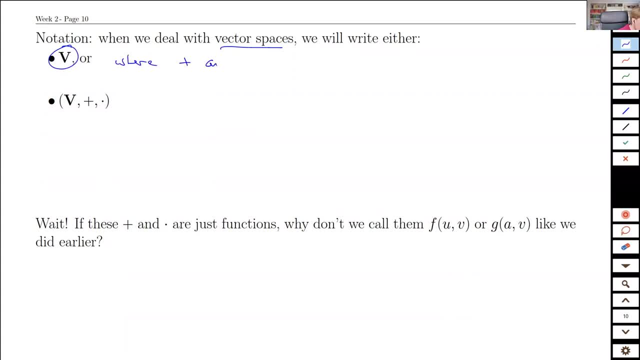 This is where the plus and the dot scalar multiplier- So addition again- And scalar multiplier Multiplication Are left to context. And so, for example, If you said the real numbers, we're going to assume that you mean, unless otherwise stated, that plus means the regular. 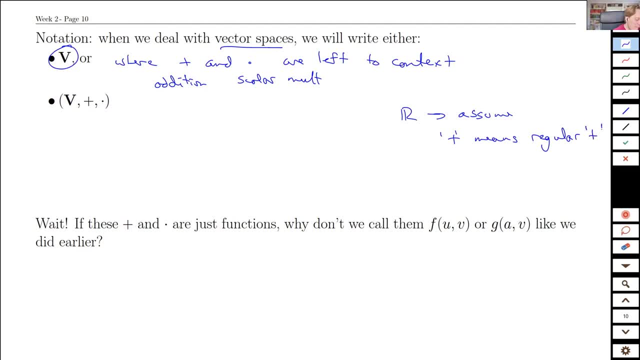 Since grade two, regular, plus The one that Exactly Left to context. What else would you do, unless you define it differently? You're going to add your numbers like you usually add them. You're going to scale or multiply real numbers, like you'd expect as well. 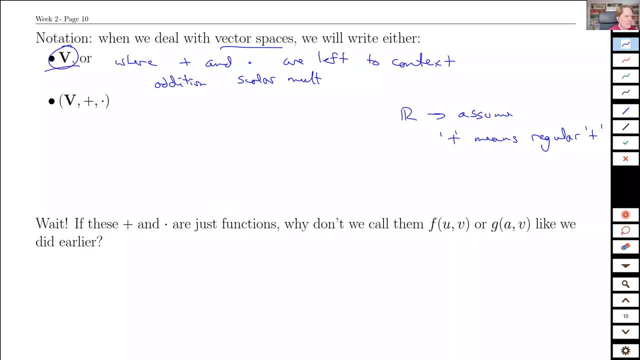 So pretty much that applies to R, to RN and C infinity, Because those all have fairly standard definitions of what we mean. We're going to add real numbers. You know how to do that. I know how to add vectors: two-dimensional, five-dimensional vectors. 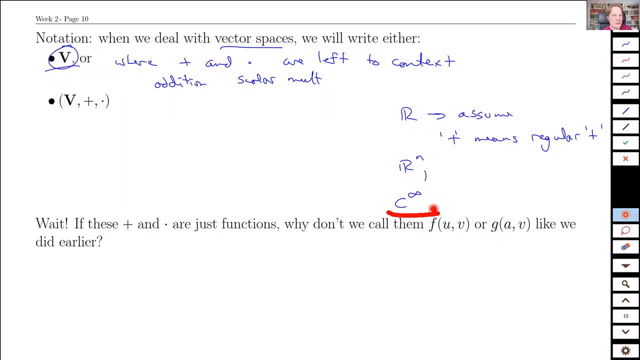 You know how to do that and scale or multiply them And functions. you've been doing that all over the place in calculus last semester and this semester. So for those- pretty much those big three, those are the ones that we just pull them out and say we know how to do that. 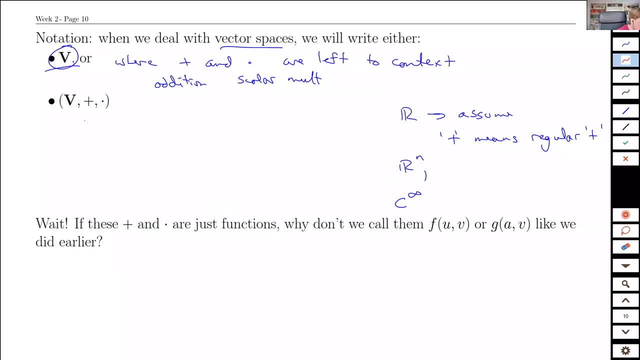 Just pull them out and say: we know what you're talking about. If it's not obvious or there's any ambiguity, We list these explicitly. List these explicitly If there is a risk of ambiguity, And it's always tough coming in here. 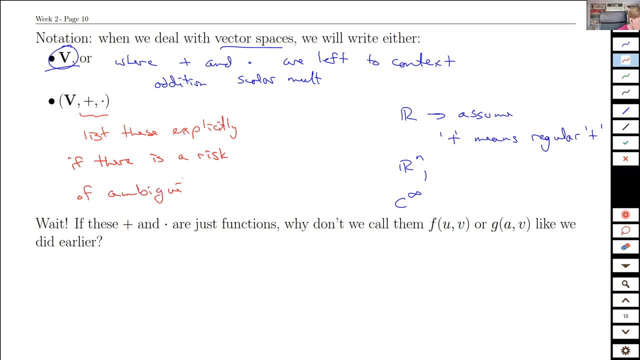 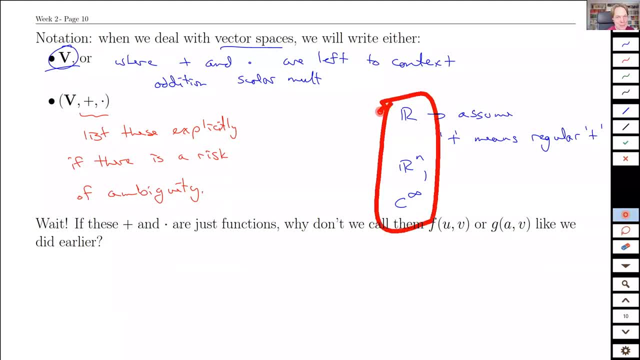 Pretty much these guys. we won't spell out the rules because we kind of know them, Anything else. if there's any doubt, we'll try to be over specific and make it as clear as possible. So one little sideline- and this actually gets to anyone who's done C++ programming back in the day or any other programming language where you can use functional things. 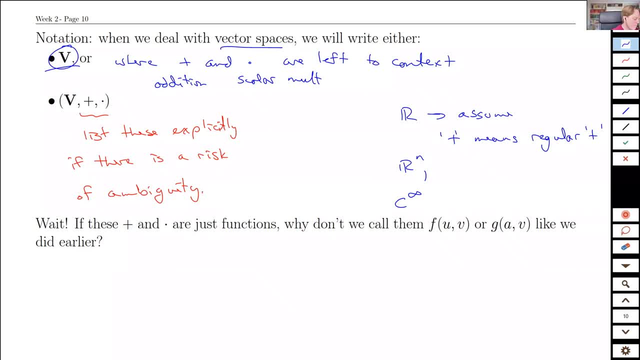 Something that it's like Observable 선생님 who writes on ed Trevor- and we've done this a couple of times, I think theη take notes on it. If all of this doesn't seem to work, then we simplify it with the Right Salve. 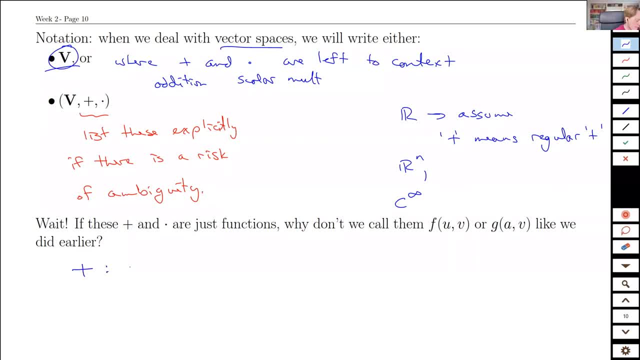 So you don't have any wird to use it with for a bee tasty thing, Because they're just not going to do it. It's just like I don't want to build a, Really know that was coming up. I think we've done a really good job. 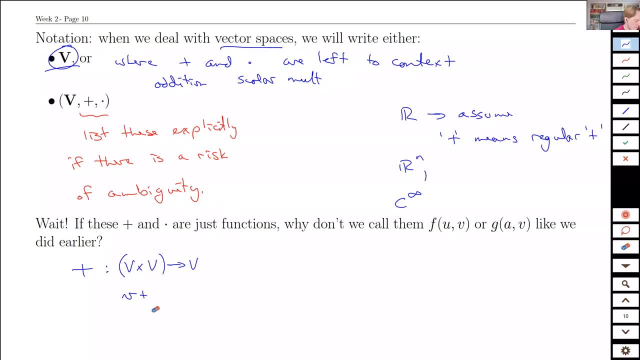 Here we go, Here we go. So if I show you this slide that the solution was not functional, then this is a way to roam around Whatever the need is. If all these things were slightly multi- quandtrull 900,- this would naturally happen. 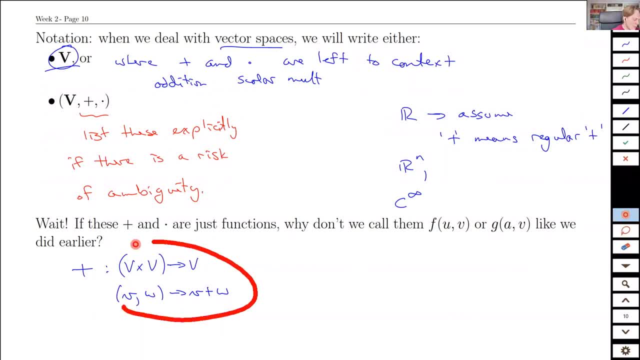 I recently read a text that it goes back to what you call theIB bastante complex differential. that's all great and all, but it's it is a function. we don't ever say that, really, when you certainly don't say it to the people in grade two learning about addition. uh, but yes, it's a function. 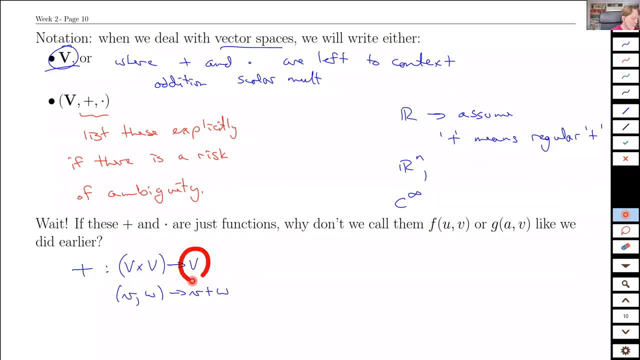 that takes two individual input values and maps to a single output value. so we could call this a function on v, cross v to v and just define it all the same way: um, vw. and the question is: well, why don't we, why don't we just, why don't we use this f notation instead? 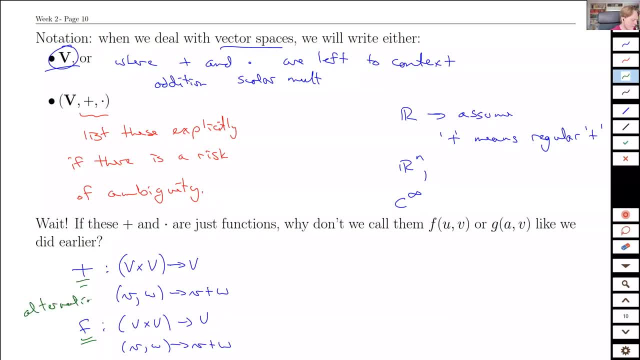 so these are perfectly valid alternatives and, honestly, it's mostly because of, i think to me it's more of the muscle memory, uh, or just the identifications. also syntax, it's easier to read. there's a whole host of reasons. easier to read: three plus four versus. 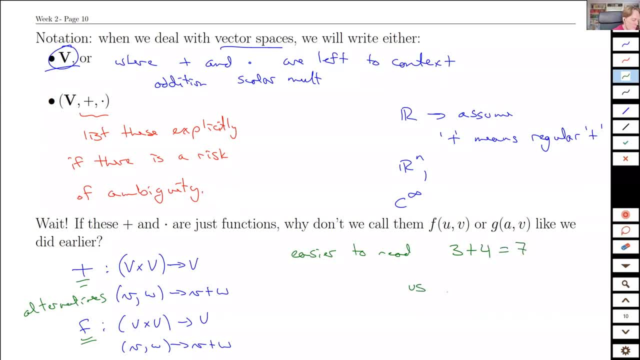 you sorry, three plus four equals seven versus- let's call it- the f function of three, four equals seven, especially when you get to distribution and stuff like that, uh. or if we said if f was our addition operator and g was our scalar multiplier, if i wanted to say four dotted with three plus. 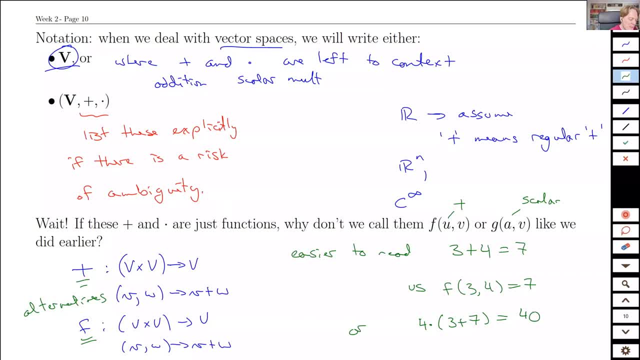 seven, that's 10, that's 40. if i want to do that calculation, it's really easy to read it out like that- versus g, g of four, so that's my scalar multiplier. and then f of three and seven equals 40. this just feels hard and weird and odd and 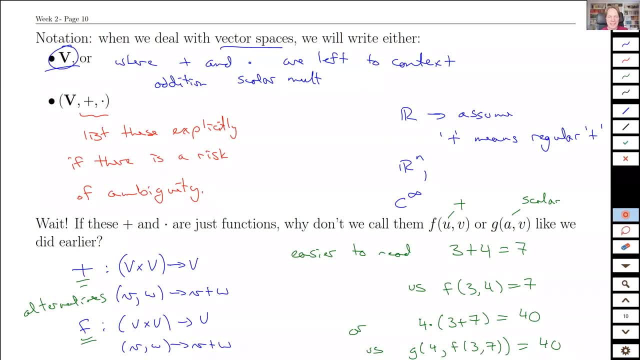 it isn't necessary. we have these lovely symbols, but just recognize that they do follow all the rules of functions that we introduced last week. the every input has to have a valid output. um, we talk about bijection and surjection and things like that. it just looks nicer if we write it like this than if we use. 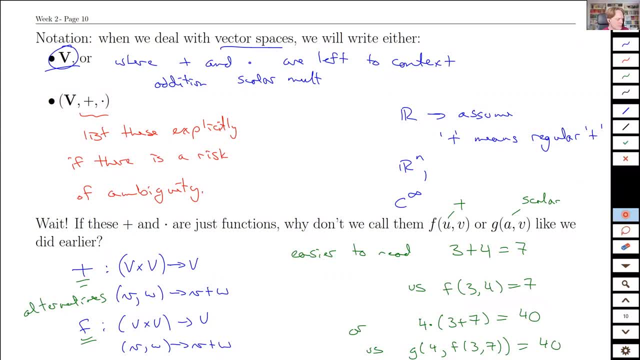 actual function notation from calculus. so just raising that issue there. uh sorry, i'm finally looking at the chat. i apologize, i'm here, right, so maybe. uh sorry, i'm just on two different computers here, so it's a little more meta than you might expect. the short answer is: if you're attending one section, it's better to switch to a. 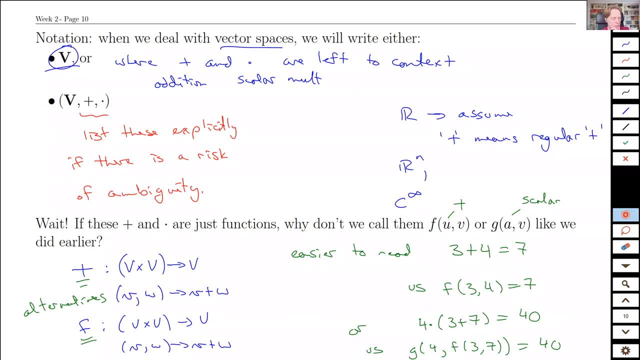 section. so we're allowing students to switch if they have conflicts or, you know, time zone, things like that. we'd rather just switch you to a section, so actually it's probably better to do that in the meantime. I'll post these notes when we're done. 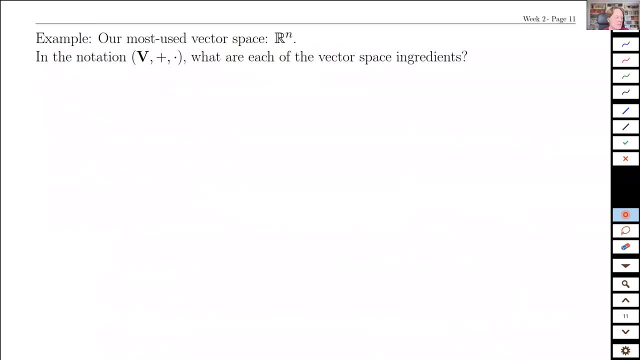 Alrighty, Okay, so let's talk about a vector space. that we're pretty comfortable and make this explicit. And so Rn is an n-dimensional vector of real numbers, right, If we say R2, that's x, y, plane, it's a pair. every element is defined as a pair of real numbers. It's R3,. 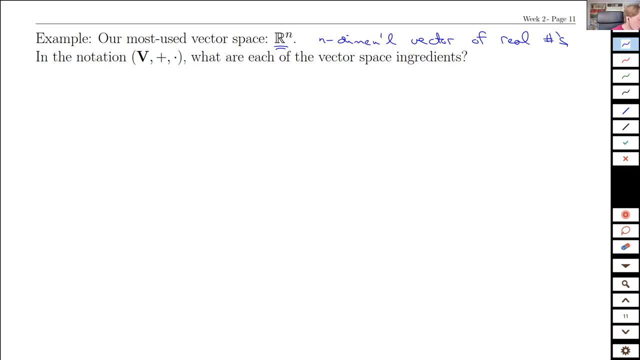 we can have a set of three real numbers where the order matters. All right, so our set V is the Rn set. So the set building block is that sorry Rn, Where each x that's in V, which isn't the same thing as Rn. 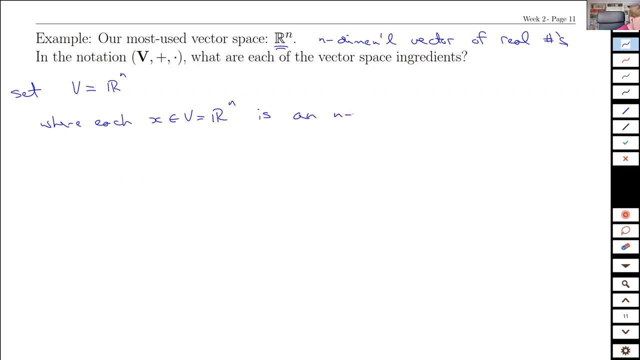 is an n-tuple of real numbers. For example, our x would be an element of some a. usually we give a subscript here: a1, a2 out to an, where a1, a2 out to an are all single real numbers. So notice: this is just regular reals, no dimensionality to it. 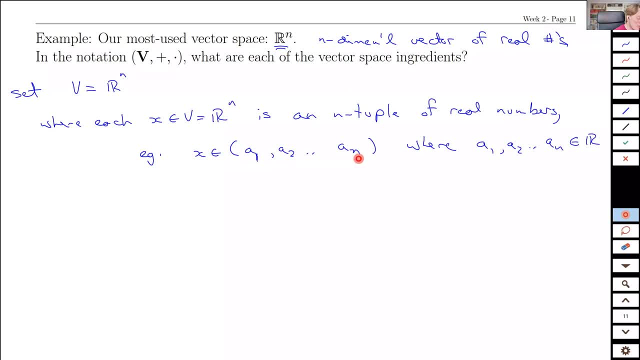 or one dimension, And x is the conglomeration of those into a vector. The plus is the regular addition that you'd expect on vectors, But how do we formalize it here? It's going to map from Rn, cross Rn and again this is the input set. 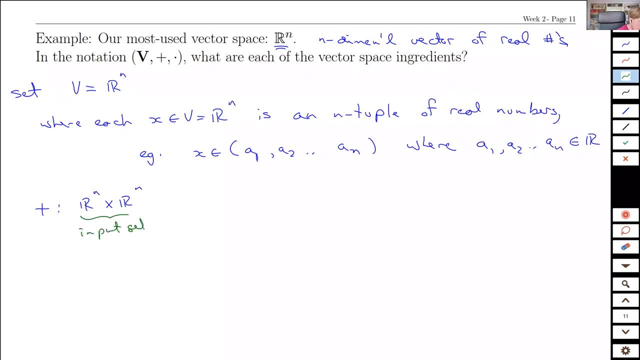 which is equal to a pair of vectors. So we add, but only add pairs of vectors, not single vectors. Then we get an output which is a single vector back. Output equals a single vector back, Also in Rn. I'm not going to state that just for brevity here. 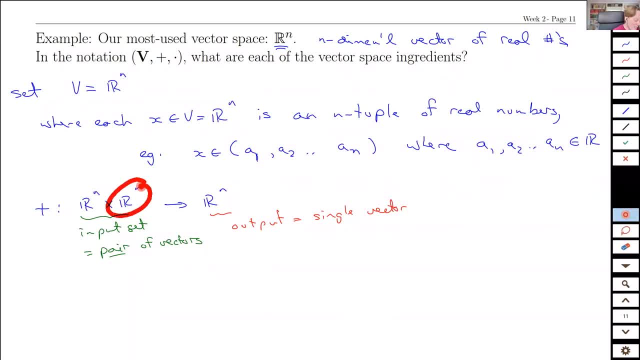 but it's important to recognize that I'm taking two vectors of the same dimensionality, I add them. I get a third vector back that's of the same number of dimensions. And the way that we add this explicitly is if we'd have an a1 to an. 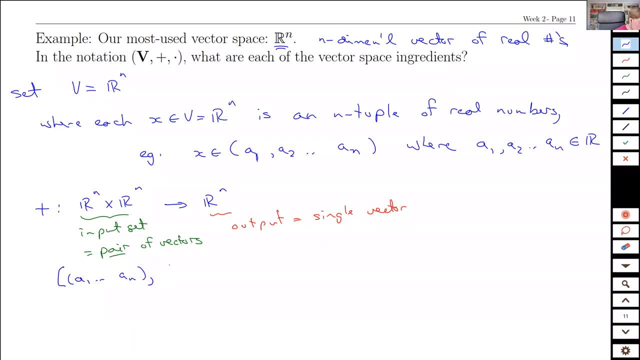 Now we're getting that vector back And we're building a little two-tuple out of this. of the two things I'm adding, b1 to bn. That's going to map to a1 plus b1 in the first component, a2 plus b2 in the second component. 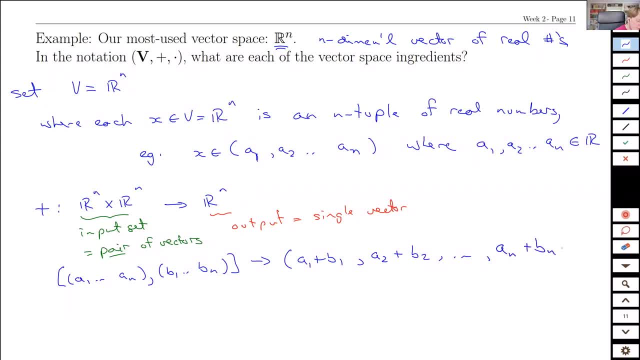 and so on, all the way up to the addition. there And again, there's context here. Each of these is the simple real number. We've gone from hey, what do you mean by adding vectors? to adding just two simple real numbers. 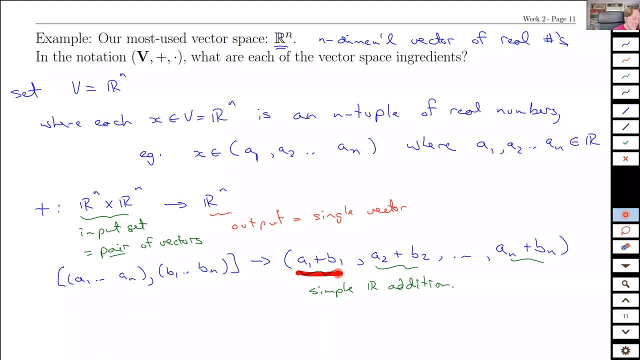 and that's what we know and love, and we've used the standard addition operator for that. So each of these guys turns into a regular, just simple real plus simple real, and we can do that. calculation Would n have to be the same number for both the R to the n's for that. 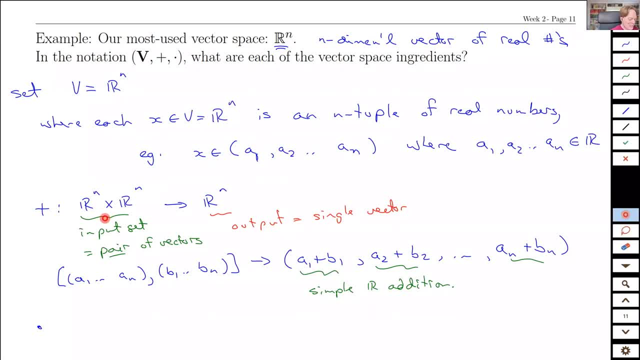 Absolutely. It wouldn't make sense, just in geometry, to add a two-dimensional vector to a three-dimensional vector. And the same thing here is true for defining a vector space. It is fixed what the dimensionality is up front. So we do this in Rn, we talk about Rn but we think of it as a specific. today it's 10-dimensional. 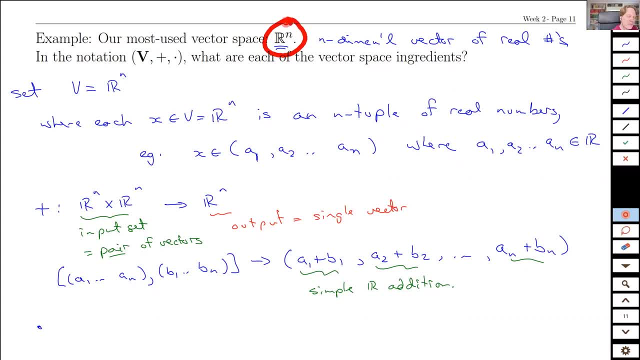 Half an hour from now, I'm going to be looking at three-dimensional space, but we keep it fixed within one application or context. Does that answer your question? Yeah, it does. Thank you. Okay, awesome Thanks, And yeah, do feel free to unmute. 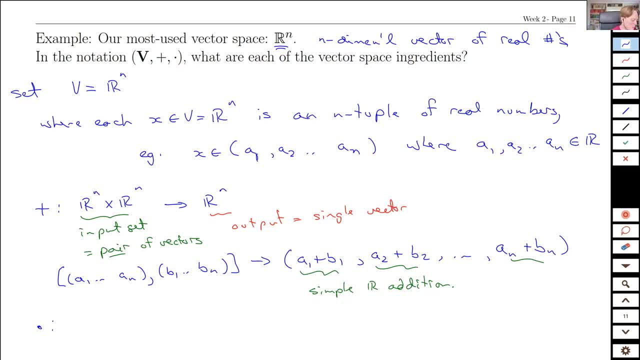 I've got a pretty good eye in the chat right now as well, so it's not crucial, but whatever way you feel more comfortable with. So in the question of would there also be an a1 plus b2, we could define that. 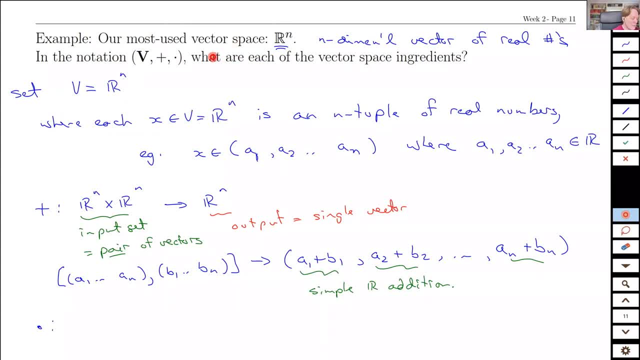 So here we're working with the vector space that we know and love and trying to figure out what are the rules that we usually work by. We are going to see the same vector space shortly where we change the rules and use different rules for maybe a good reason for a certain application. 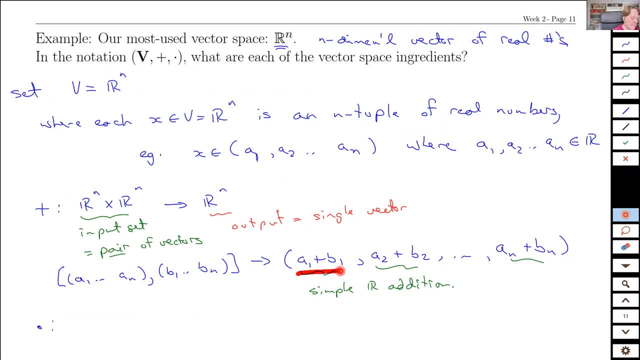 So right now we're just talking about the default rules, and the default rules are definitely: add up the x-components, add up the y-components, add up the z-components. That's how we usually do vector addition and, as we're going to see in a second 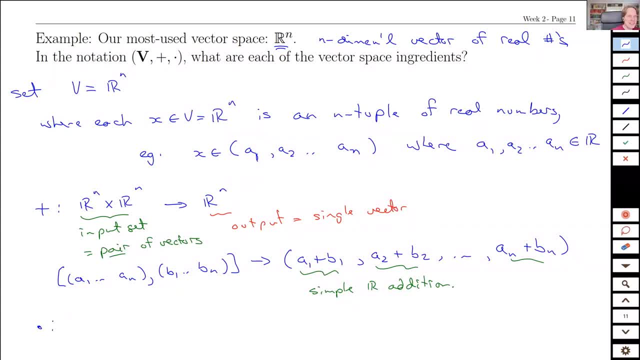 scalar multiplication for Rn. So this is the common way that we have been doing: vector addition and scalar multiplication. So Okay, The scalar multiplication. notice that this first R here is just a single R. It's R to the one, and then we take that times Rn. 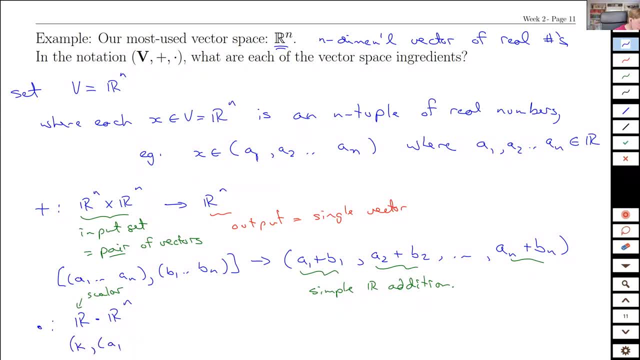 And so let's do this as k and our vector a1 to an. That maps to a new n-dimensional vector. So again, this and this are the same. If you take a two-dimensional vector and you multiply it by five, what happens? 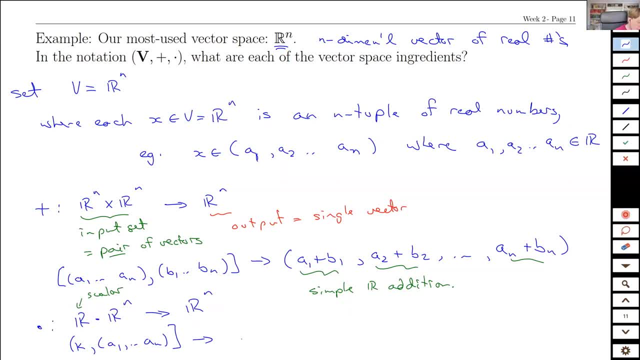 You get another two-dimensional vector back, And, and, and, and. The basic way that works is that you take the scalar multiplier and basically you distribute it in. Distributivity is sort of what I think of when I see this. 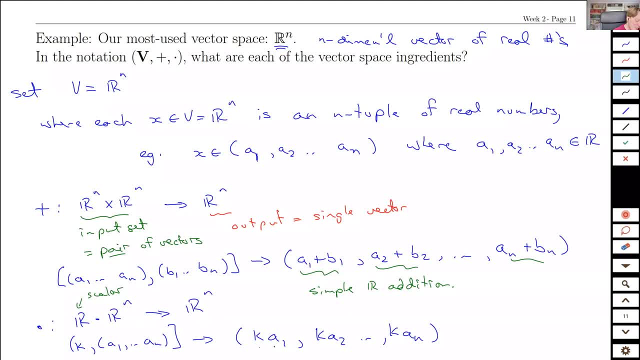 Where now we have, each of these a's is just a real number, The k is a real number, And so this is just regular or simple real number multiplication. Okay, It's kind of the easiest thing we could think of that does what we sort of expect. 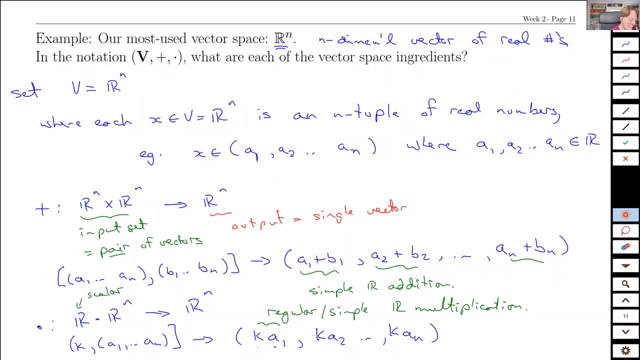 If I take a vector- sorry, a vector- and I multiply it by a scalar, I'm just multiplying each component individually by that same scalar. That's the same. That's how we're defining scalar multiplication here. All right, Again, you do all this. 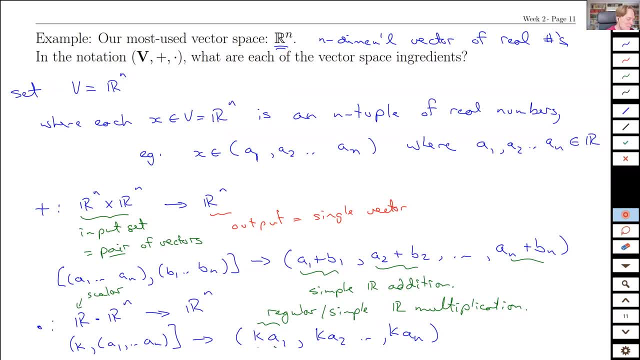 This is not, this is not the interesting part of vector spaces yet, But it is trying to give you some context and remind you. yeah, there are rules. We don't really state them, We just kind of illustrate them and have you figure it out from examples. 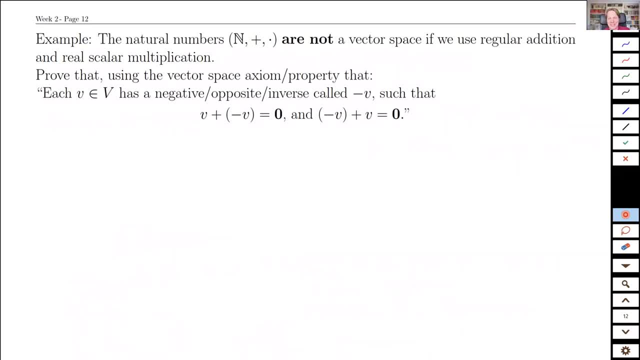 But these are the rules that we use. What would be an example of not a vector space? Well, let's take a look at our natural numbers. So our natural numbers, remember, are the set of 0,, 1,, 2,, 3.. 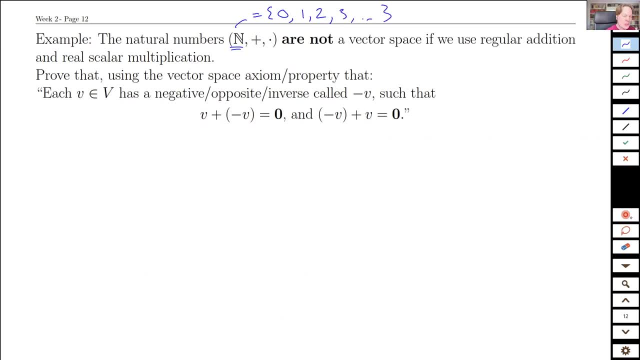 They do not have the negatives. The negative numbers are in that zed set, the integers. So let me just take a step back. So we're going to talk about the natural numbers And we're going to define this As sort of the regular addition. regular addition. 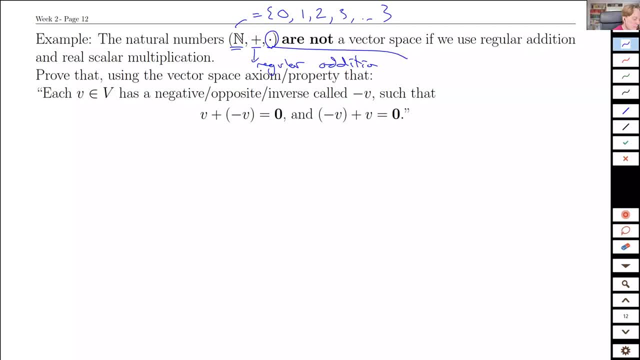 And we're going to talk about the real scalar multiplication, scalar multiplication, But it's important to notice that this is with real numbers. When we've been talking about a real vector space, we've been allowed to use any real number to multiply the elements of the set. 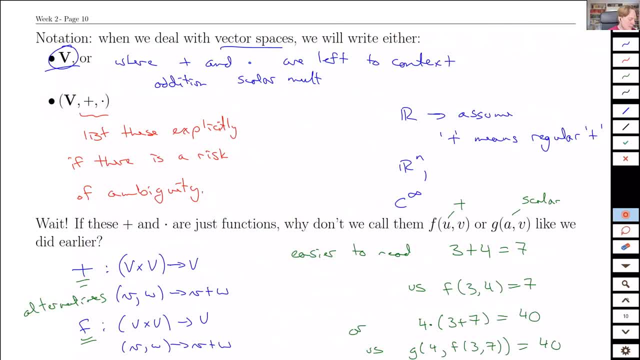 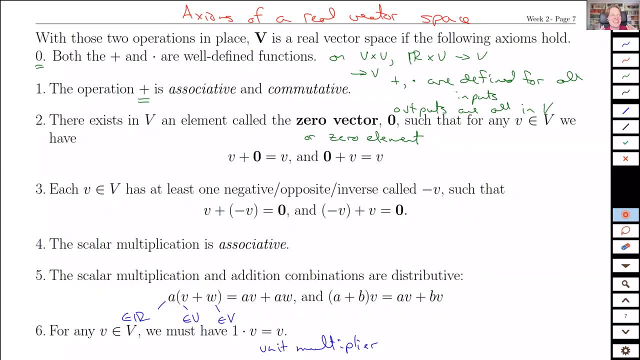 So let me go back here And what we've just done is put together a set. We said: hey, I'm going to look at the whole numbers, the natural numbers, and see if they fit all these rules. Can we define these things as functions? 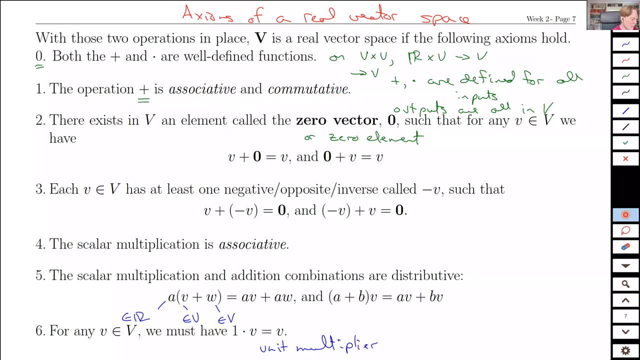 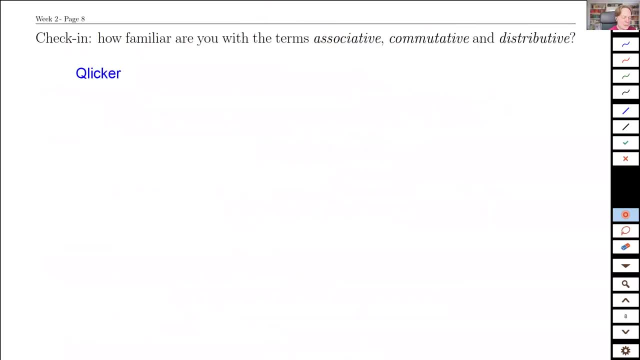 Is the plus operation, associative and commutative. It actually turns out that is. Can we build a 0 vector or a 0 element And can we define? do we satisfy all these rules in this set And unlike so we've shown this is basically true. 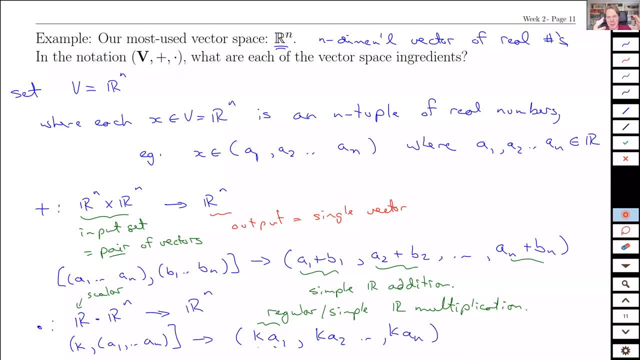 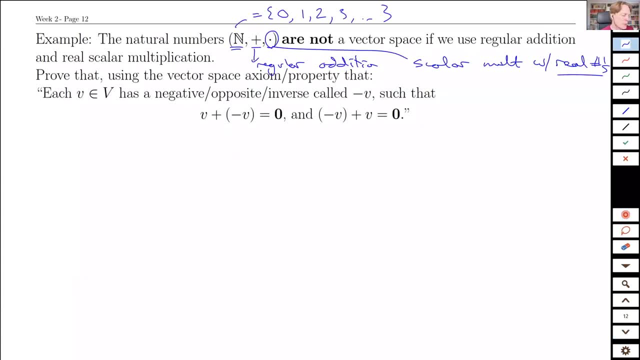 We had the intuition. This is true for the real numbers. It's true for real number in vector form, Rn. It's true for continuous differentiable functions. However, it's actually not going to be true. We're not going to be able to satisfy all those rules for the natural numbers. 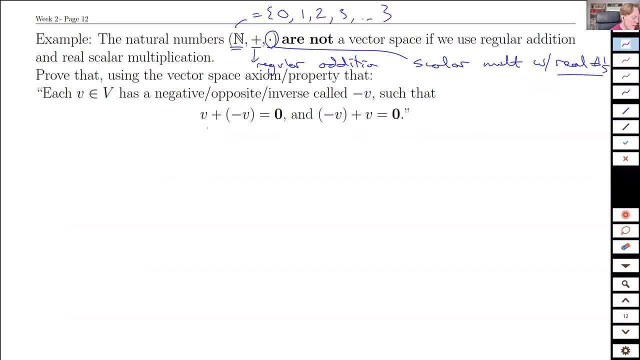 And one glaring hole we can see is we're supposed to be able to build a negative version of every number, And so we should be able to build. We need to find, For example, v, so let's call it minus v. The notation is a bit awkward here. 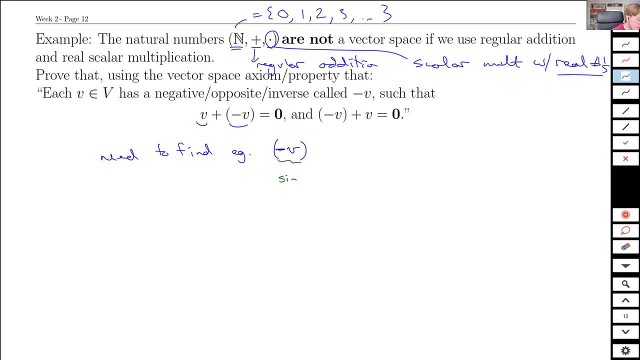 But this is a single element, single element of the natural numbers That satisfies I should have said here. Here's the example: Eg 3.. Plus this element equals 0. And you have the obvious answer, which is negative: v is going to be minus 3.. 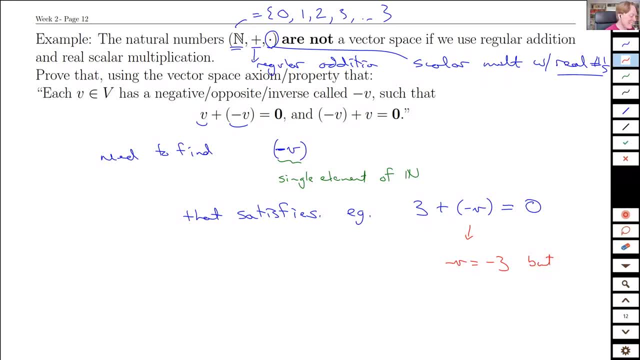 Oh wait, But what exactly? The problem is that negative 3 is not in the natural numbers, And so that's a problem. And so you can go hunting for other answers, but you know there's no other answer. The thing that you add to 3, that gives you 0 with the regular. 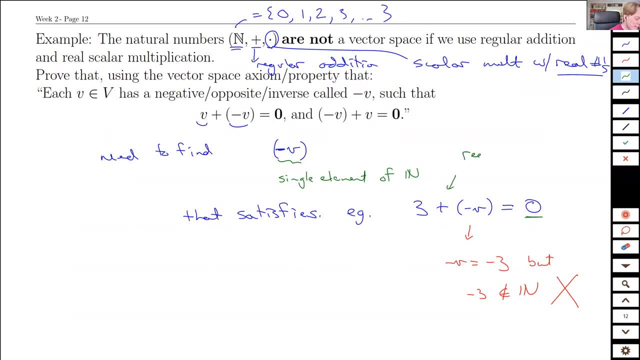 And here we have to say, okay, are we using a regular or simple regular? This is actually sort of real to real addition. But we can also say integer addition, They're the same addition. We hit the snag that we can't find a negative for every quantity. 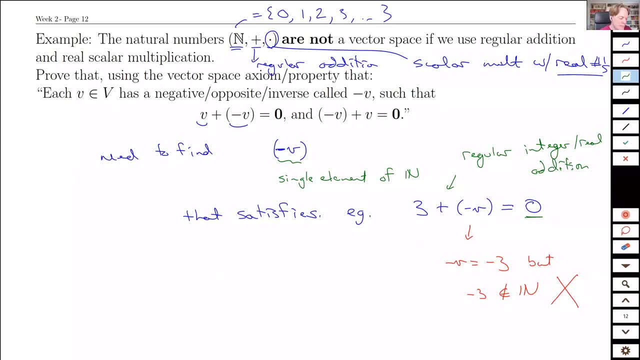 There's no additive inverse for everything in my set And that's all it takes is 1 to break the rule. So as soon as I have 3 here and I try to find its additive inverse, what would cancel it in an addition sense? 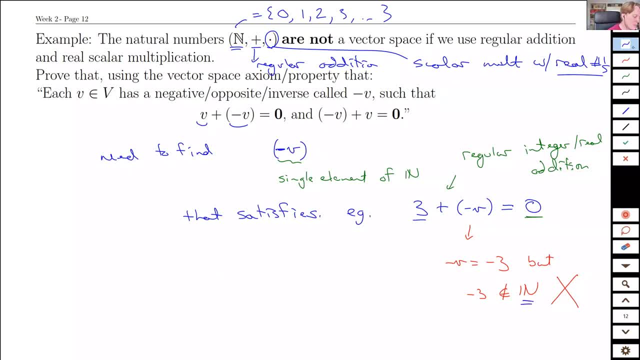 There is no number in our set that we're allowed to use. So this tells us that for n there exists x's that are in n. Let's call it v. it's the same thing here: v, for which there does not exist an additive inverse. 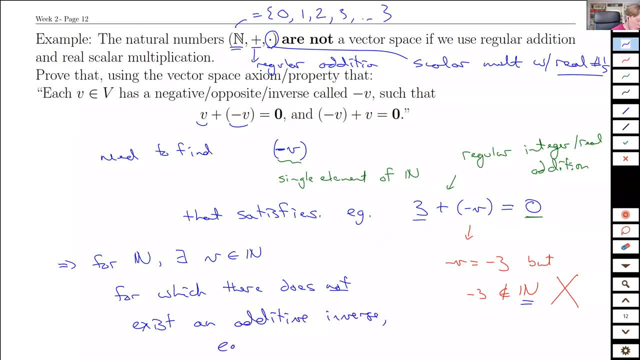 And then we can make it concrete. We can say: eg 3,, which is a natural number, does not have that additive inverse, But it's worth knowing that's just one little failure. I mean the conclusion is going to be the same. 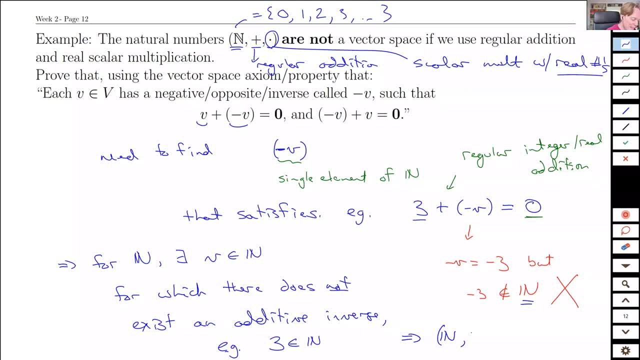 The natural numbers, especially with our usual plus and scalar multiplication, is not a vector space And not a real vector space. And I'll just say this explicitly here: Sometimes we get sloppy and we don't talk about real vector spaces. Again, context is: if we haven't seen a complex number in a long time. 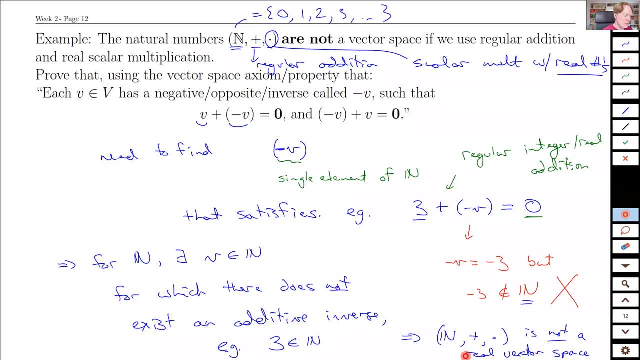 vector spaces are real vector spaces. We just kind of assume that as sort of the default, So I may slip up on that. I'm going to try to keep saying real vector spaces, But if I just say vector space, the real is the default choice. 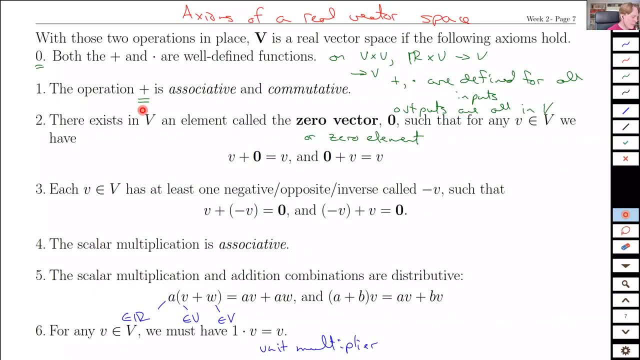 So, going back to our list of things that we need for this, it turns out that the natural numbers here actually are associative and commutative. You can swap, adding two integers or whole numbers, and that's fine. The association is fine. There is a zero vector. 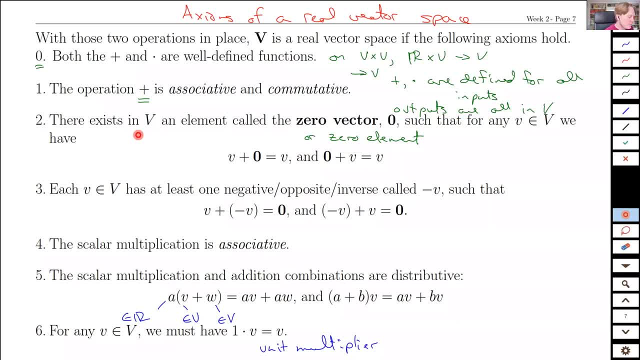 There's a zero element, The number zero is in that set, so that's fine. So you can have a whole bunch of things that are satisfied, but all it takes is one to break things down As soon as one of these axioms is not satisfied for a set. 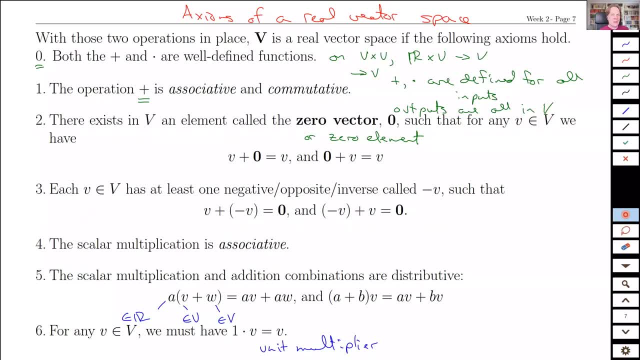 then you're like: no, that's too bad, This is not a vector space anymore, because we're going to use combinations of all of these. We're going to use all of these things to prove a bunch of ancillary properties. So if you're a vector space, you have all of these. 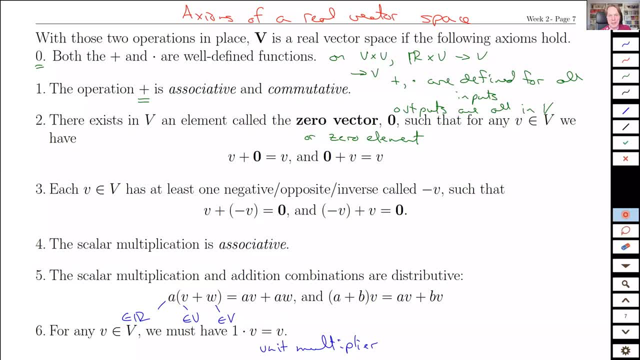 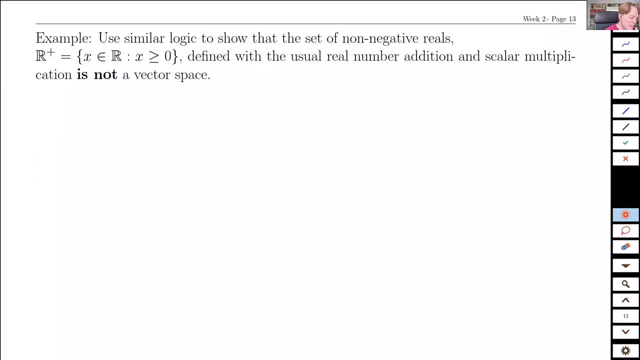 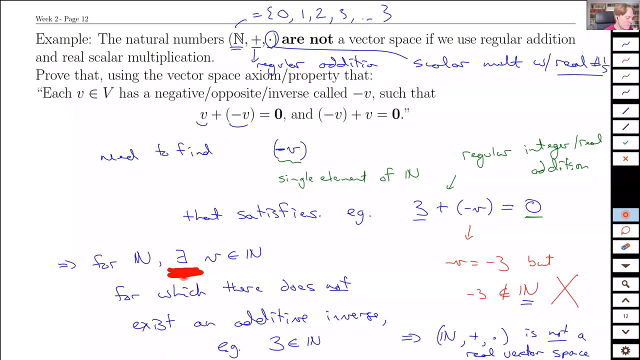 If you break just one of these rules, even just a little bit, then you're not a vector space. That's our logical framework we're working with, And yet that backwards symbol there exists. So being deliberately explicit in using that, because that's a very common short form that we use in math. 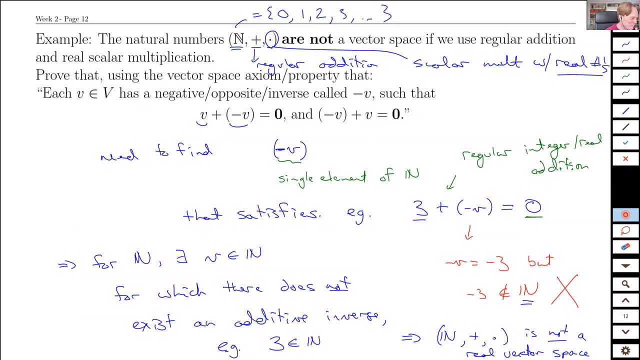 So it's a backwards capital E and it stands for there exists. So we're going to have something not associative and commutative? I think we might. Now it turns out those are really. You have to do some weird stuff to break associative and commutative. 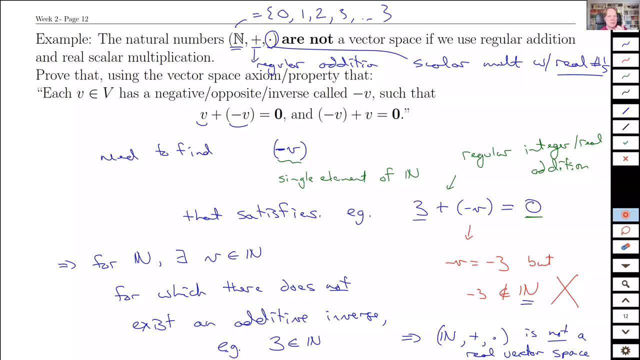 So I don't think we're going to stumble across that For most of our examples- the zero vector, zero element being missing and not having additive inverses- those are usually where we fall over, Just because it gets so weird. It's the kind of thing like: why would you do that? 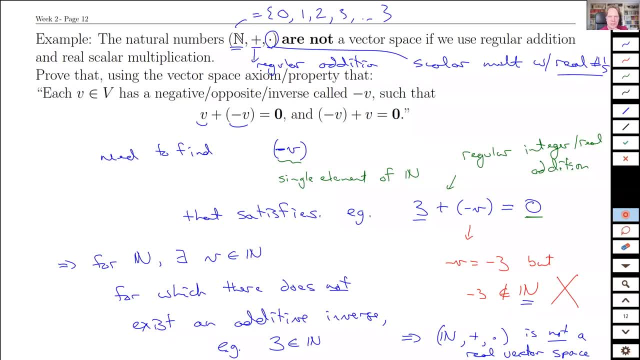 So, yeah, we're not going to see so much about breaking associativity and commutativity. We're just not. It turns out they're important and commutativity you might see by the end of the course with matrices, but the other ones are going to be the ones that typically trip us up. 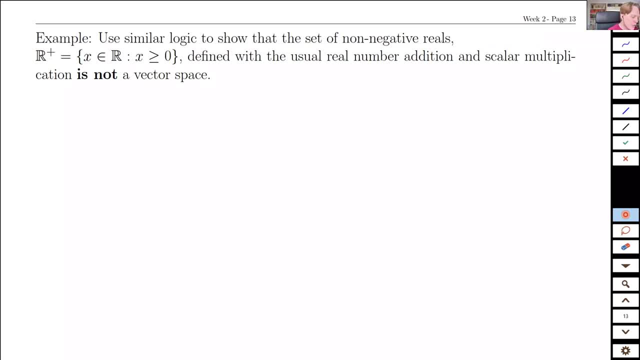 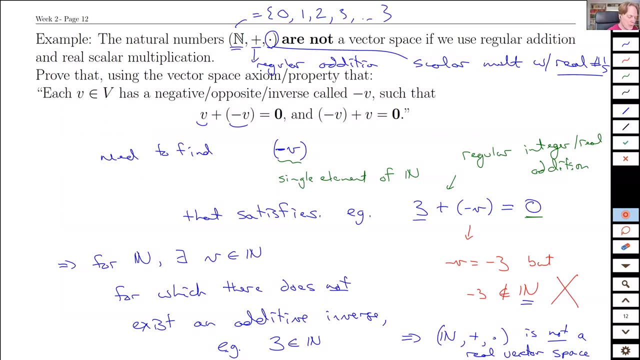 Alrighty. So similar idea If we take a look at the not natural numbers. So here we have the natural numbers, which automatically are just the positives and zero. We can do the same thing with the reals, with a little plus sign here to indicate. 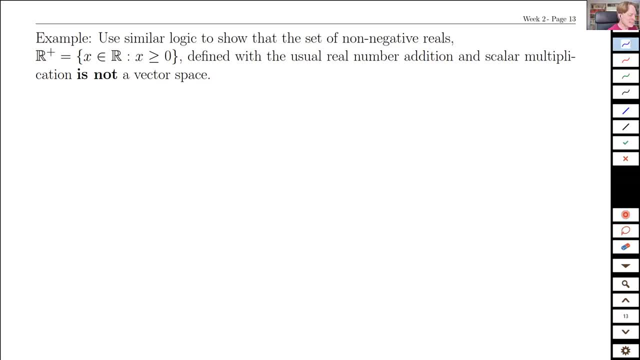 yeah, it's the reals, but We're going to be a little finicky. Not all the reals, just the positive numbers and zero. So this is our plus is zero and up, And of course we have the same problem: that there is no additive inverse. 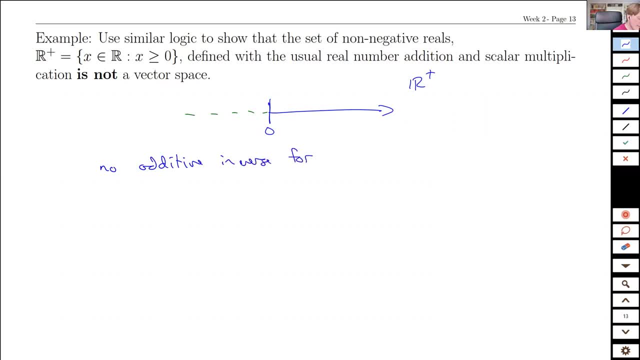 inverse for EG 3.792.. Which is in that set, Because 3.792 plus- let's call it some- minus V here again has to equal zero as no solution. No solution where that minus V element is in. Let me slide this over here. 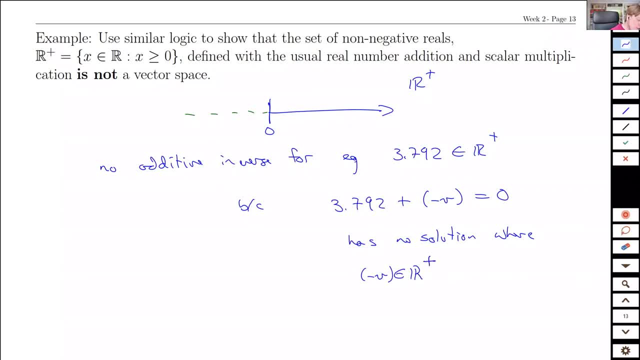 There we go, Where that element is in the set that we are looking at here. So we cannot find what we know what the right answer is. The right answer is negative 3.792.. But that element is not in the set we're looking at. 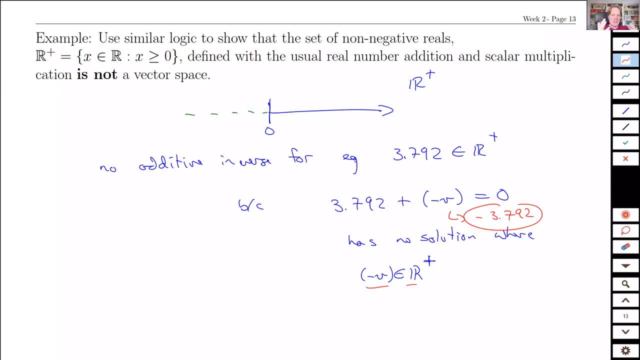 So somehow, if I add these things together or try to invert them, I get out of the set. There's this feeling with vector space that I don't want to escape the set I started with. Another example of this is that scalar multiplication is a function. 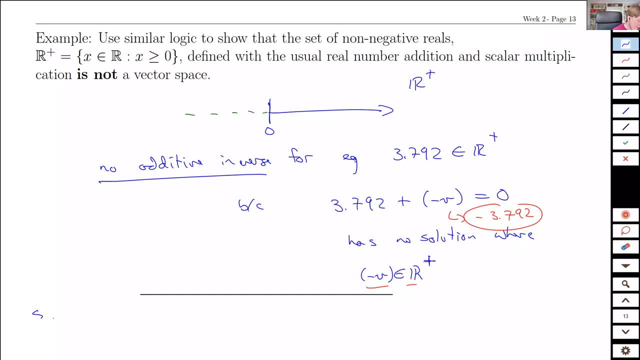 So this is violates. So there's no additive inverse. Also, the scalar multiplication. scalar multiplication with reals is not a well-defined function So I can't do it, So I'm going to use a scalar multiplication for this set here. 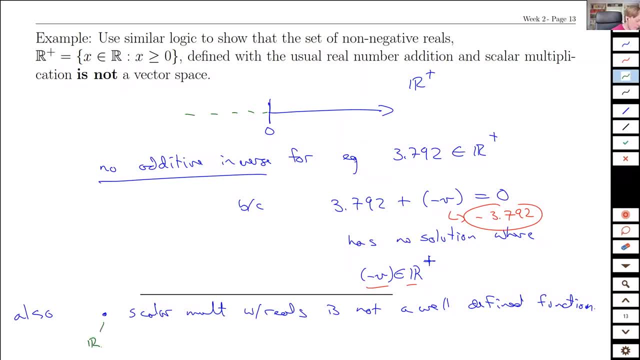 And the reason for that is the scalar multiplication can take a real and one of the elements in my set. So real multiplication, scalar multiplication, I'm allowed to pick any real I want and multiply it by an element of the set. However, if we do an example with that, like if I pick my real number to be minus 2,, 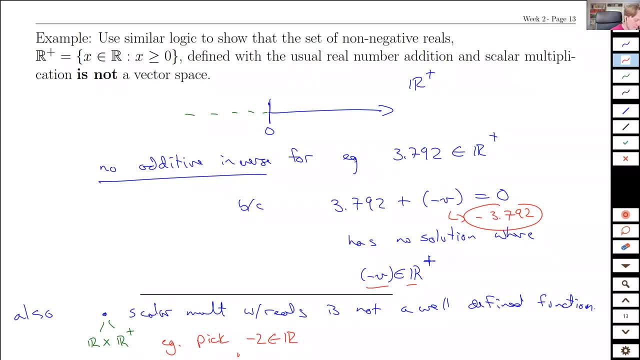 as my real multiplier. then minus 2 scalar multiplying times any v, with v in the positives, gives a value outside, outside the positive reals. If I take minus 2 times 3, I'm allowed to use 3. But then when I'm finished my product I get minus 6 at the end. 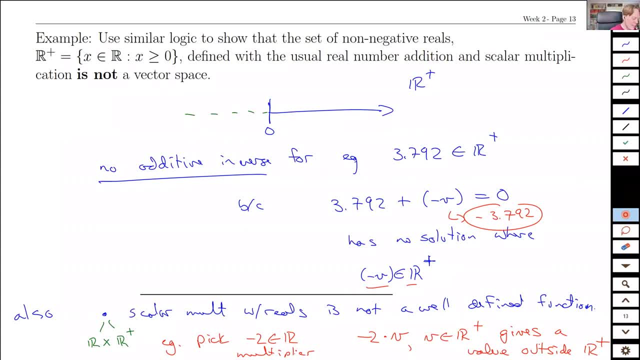 Well, that's not in my set. The scalar multiplication has to give a new element of the original set. I've got to stay within my set. whether that's the reals, the Rn Here, the positive reals, they're, somehow I need the other half of the reals to make this work. 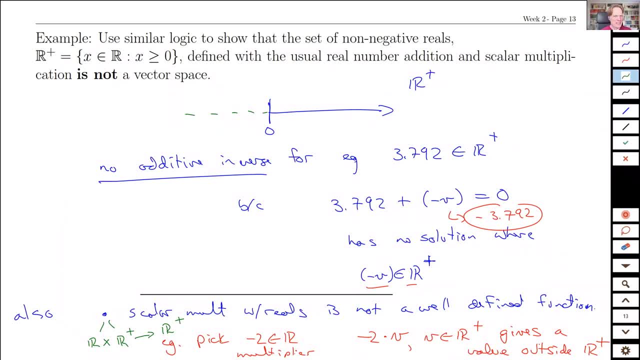 Just kind of like the other. I need the other half of the natural numbers to at least get closer to what a vector space is. So there's some idea in vector spaces of having center at zero and stuff on either side, And that's true even for Rn functions. 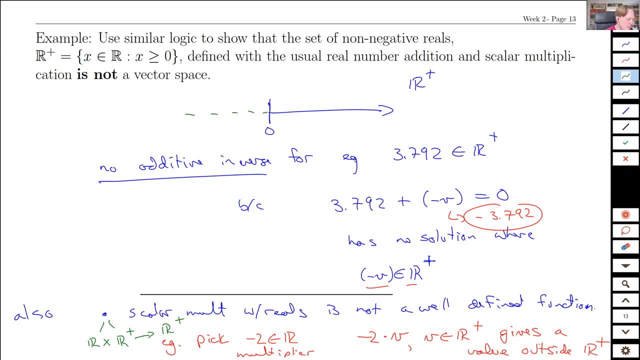 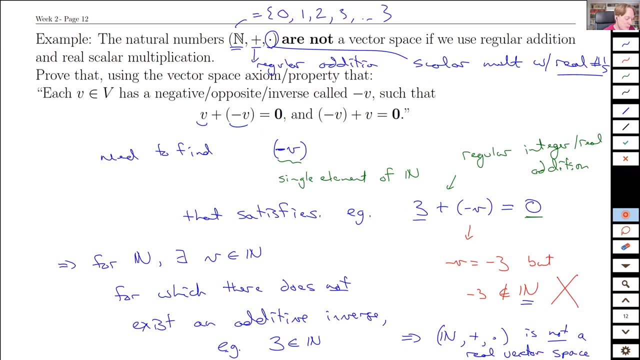 You can think of positive and negative functions in a zero thing, but you need both sides of that to be a vector space, So there's no difference at all in terms of how we handle the natural numbers for this example here. In fact, the same complaint could have been lodged against. sorry, 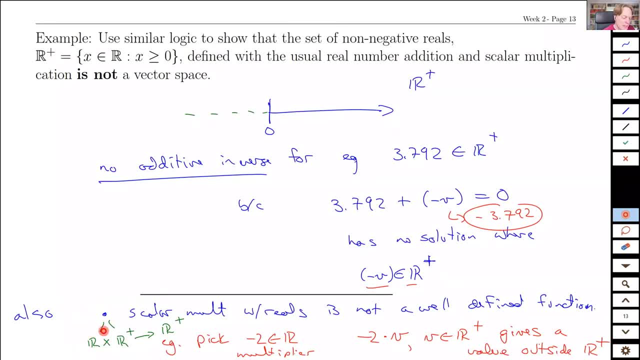 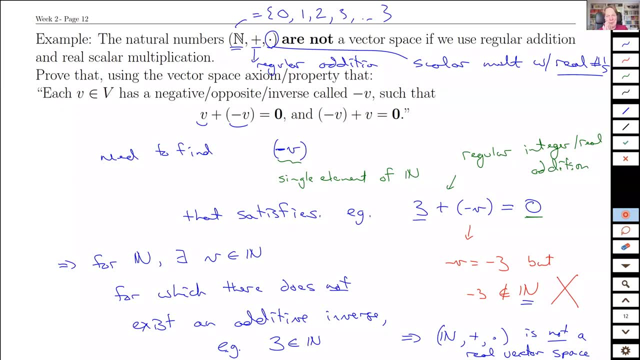 this same complaint about scalar multiplication by a real could have been a deal breaker for the natural numbers as well. So it turns out there's a lot of similarities between the natural numbers, which are just zero and up integers, and the reals zero and up. 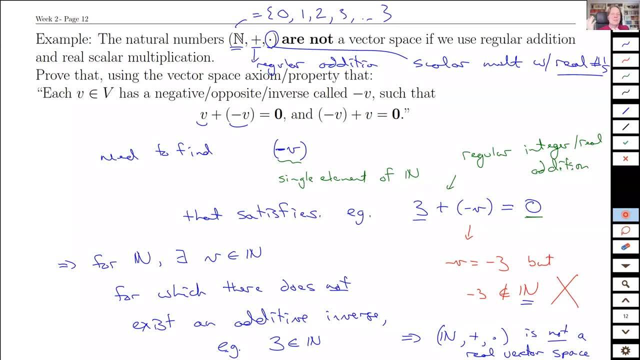 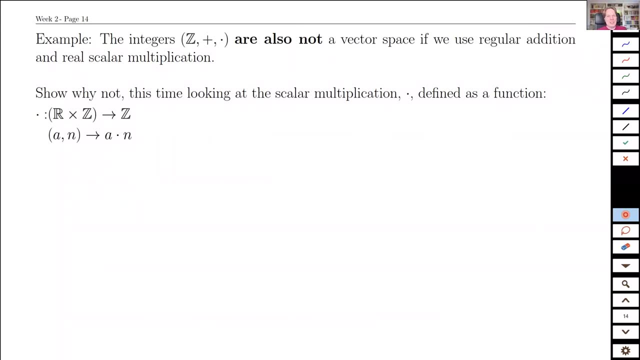 Neither of them is a vector space, for sort of the same reasons that you're missing this complement set, this negative part that you have to have to be a vector space, Just to show that it's not just the natural numbers. NASA Jet Propulsion Laboratory Bostoncom. 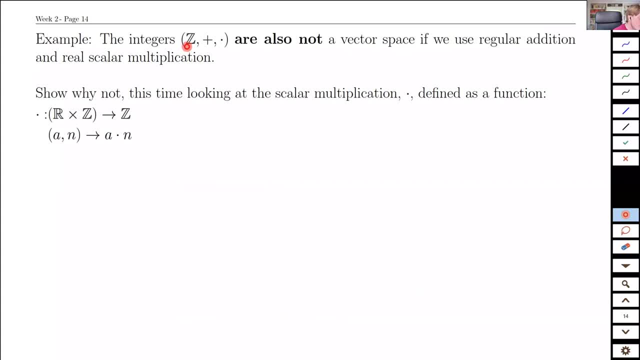 NASA Jet Propulsion Laboratory Bostoncom. negatives, though it's a little more subtle than that, even The integers which do cover the negatives- minus 3,, minus 2,, minus 1, 0, it's going to have the multiplication problem. 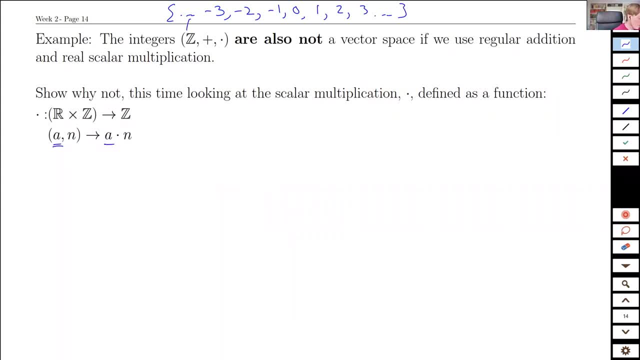 So if we use scalar multiplication for this, we're going to have a problem, because if we take an example of minus 3.7279 as an element of the reals, and let's say 5 is an element of the integers, zeds, but negative 3.79, scalar multiplying 5, which is equal to some. 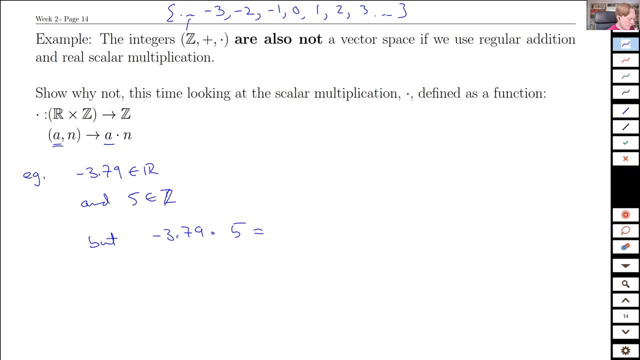 nasty number here: 3.79 times 5.. Negative 18.95 is not an element of the integers, So the scalar multiplication. again just like the last time, multiplication is not a well-defined function. Function on the reals. 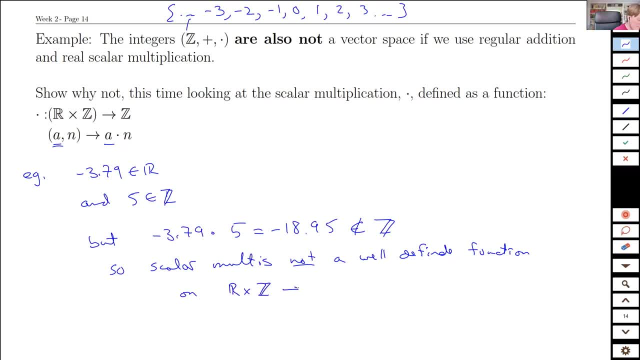 I should be able to take any real times an integer and get an integer back. Let me as, as is probably a better word here- as: So if we take a dot product, it's a scalar multiplication product- we're supposed to be able to take any real and any integer and 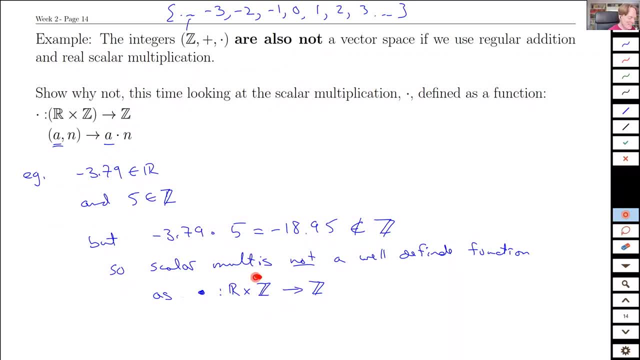 multiply them and we can do that, but it has to give us back the same kind of number that we have in our set and our sets of the integers. so we're out of luck there. Oh yes, I prefer arbitrary rather than random, so why 3.79?? As long as I picked anything, that's. 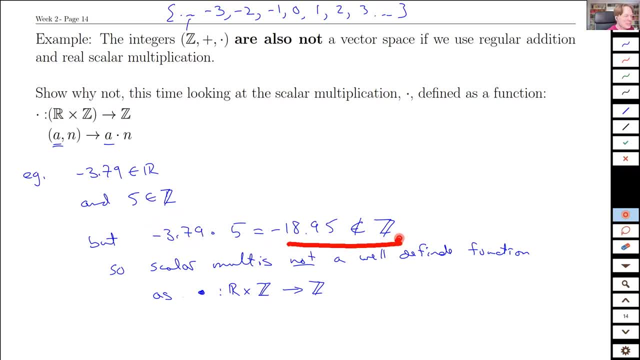 not an integer, I would get a result that is also not an integer, unless I had things worked out nicely. But yeah, we're just looking for one counterexample. If I can show one example of a real times an integer that is not an integer, then I've got a problem. And 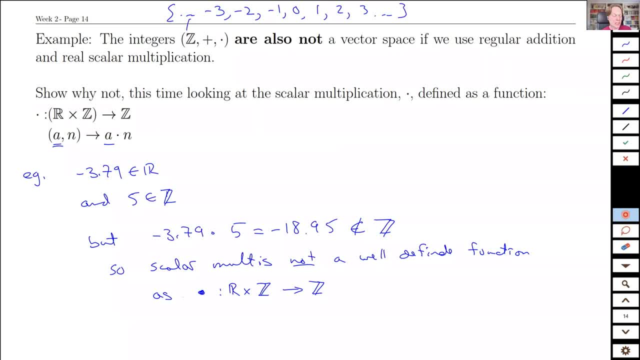 what we have there is that our scalar multiplication is not well-defined. our real scalar multiplication is not defined. There's not a vector space. This observation, this one example, counter example, shows that scalar multiplication is not a well-defined function and so the integers are not a real. 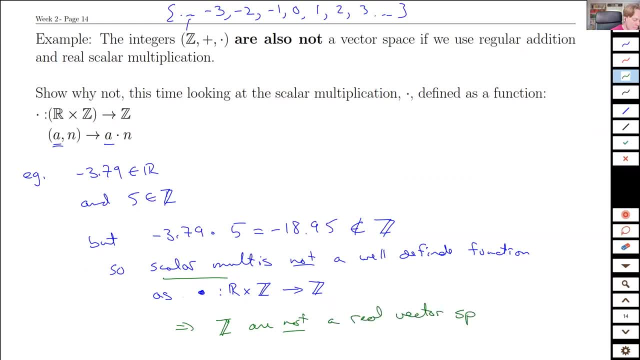 vector space. Okay, And that's despite the integers having negatives and positives, right? I mean, we, the integers, have negative and positives. Yeah, Yeah, Yeah. So it wasn't that we couldn't do opposites and adding, we also have to have a lot of. 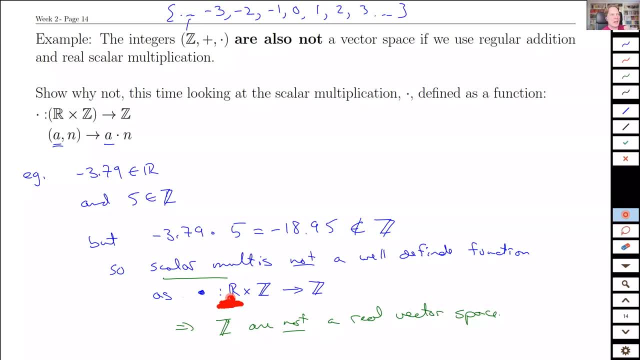 numbers. As soon as we're going to have real multipliers, somehow we have to cover all the numbers and kind of allow us to get to the numbers in between the integers. here We have to be able to get a more finely split up. 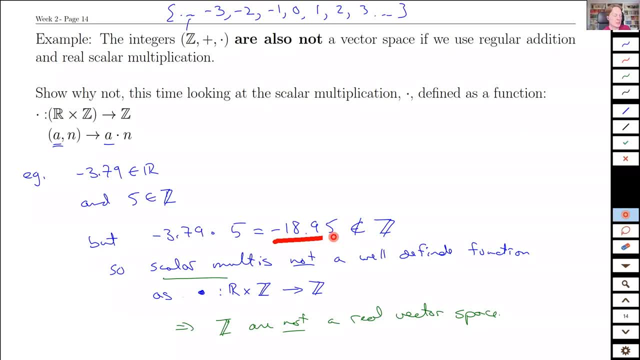 So the sets that we're looking at tend to have a lot of points in them Usually, in fact, they usually have an infinite number of points in them And they have to be kind of packed together because we have real multiplication. So, again, you'll get more experience with this as we go through the course. 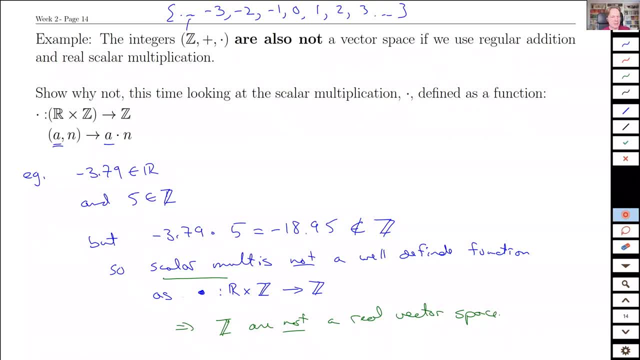 But these are the kinds of things that I think about when I'm thinking about vector spaces, sort of this continuity in them which the integers would not have. That continuity turns out to be important and it's sort of reflected by this multiplication not working with the integers. 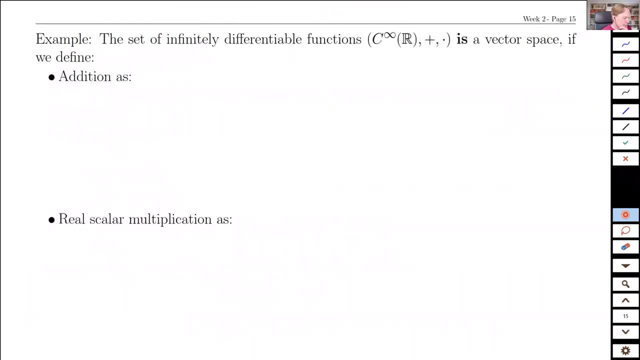 All right, 20 after all. right, I think I want to stop there. just I don't want to keep you late. So what we're going to do is we're going to do a little bit of math. What we're going to do is we'll pause here and we will do a quick little summary. 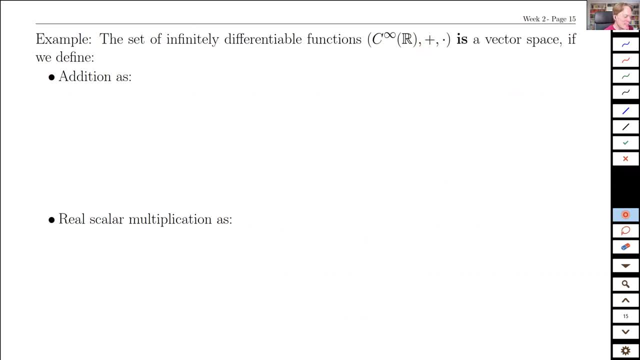 So between now and tomorrow's class we can take a look at the C infinity and think about what that meant, And what we're going to do is do a quick little summary at the end of things that we've seen that are vector spaces and aren't, and just try to get it again, that sort of intuitive feel for what things play by the vector space rules. 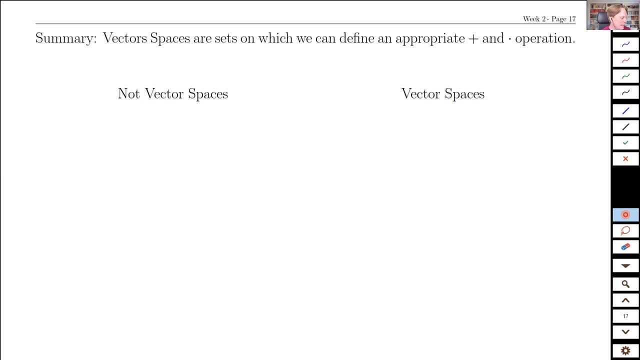 and what things don't. All right, so I'll happily stop there And again, if you have other questions, I'm happy to stay around for as long as people have them. Otherwise, enjoy the rest of your day or other classes and everything else. 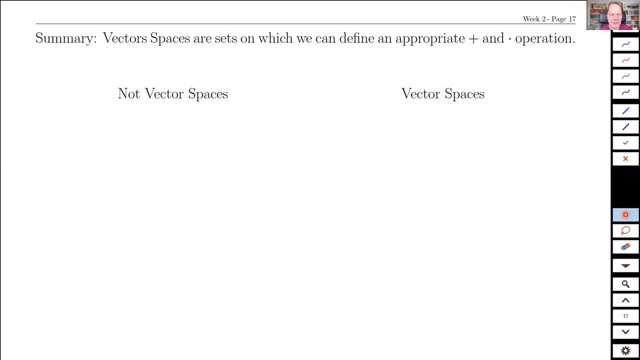 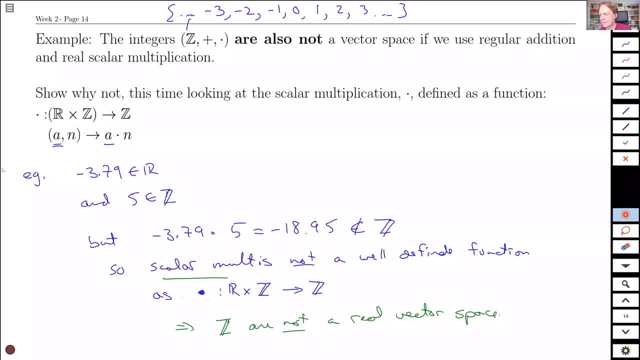 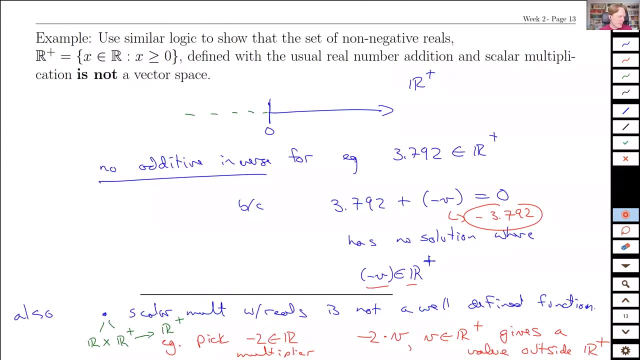 Let's look back to that last slide for those who are still taking notes, And thank you for coming. Could I ask a question about the previous slide, please? Yes, go on. I was just wondering in the notation why it says negative v is a member of the real plus. 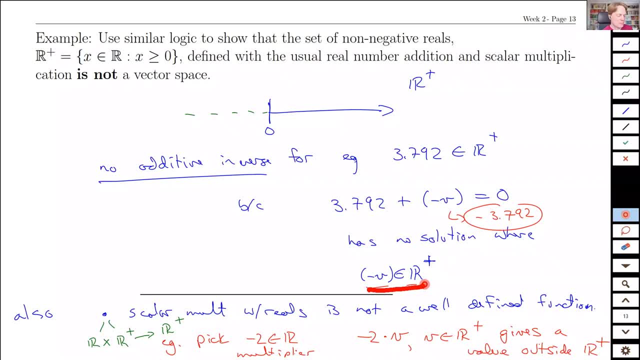 Oh, it has no solution where it is, So that's the whole sentence. Oh, so it's the same thing as saying v is not a member of r. Yes, And that real plus just means it's like that's just what you defined up there. 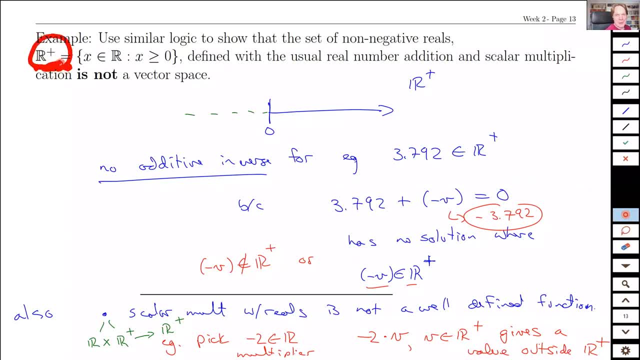 Exactly For the purposes of this problem, we said: hey, let's make up a new set and we'll give it the name r plus, because that seems more mnemonic than v. Yeah, OK, And if they were multiplying it'd be real with a dot next to it. 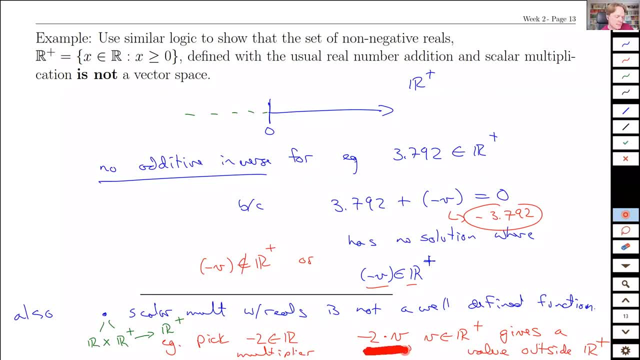 Sorry where? Oh, like down here? yes, But why is it still r plus? Wouldn't it be like r dot? Or is that just something? Oh yeah, it's your point. No, fair point. This plus was meant to indicate positives rather than addition. 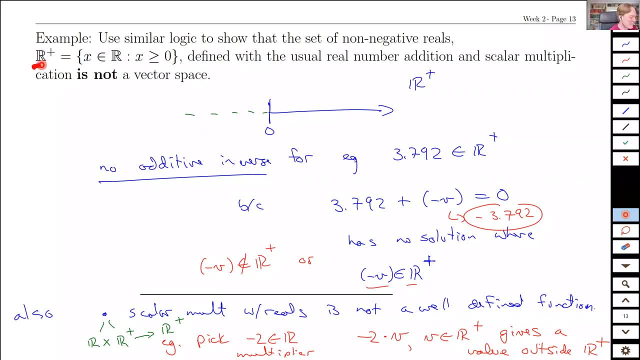 So maybe it would have been better just to call it v. So we're just taking all these numbers, That's this whole unit. r plus altogether is a set. And then we say, does the plus- unfortunately- plus addition operator work on this? 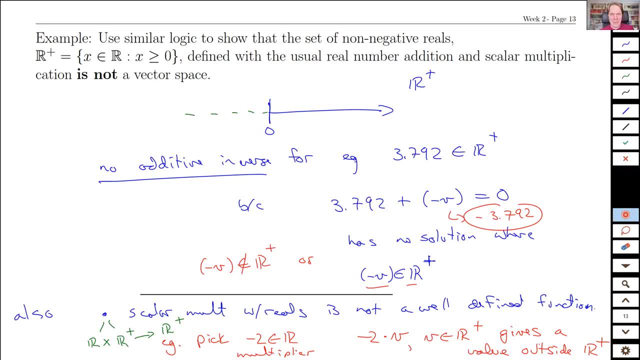 Yes or no, But it's always r plus. R plus for this entire page is the set. All right, Thank you. No, thank you for asking that. I hadn't realized that could cause confusion. No worries, Oh, I just saw Emma's question about: are we going to finish the week? one slides. 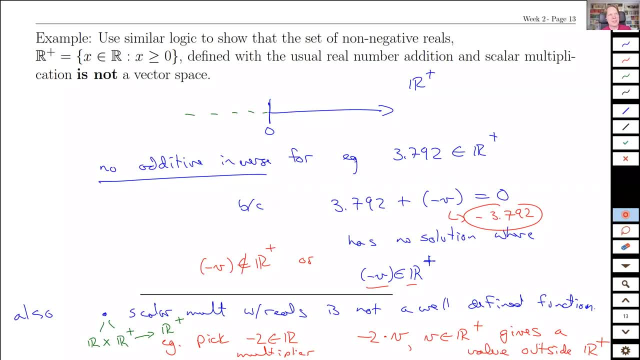 I debated that. The short answer is no. You've already solved linear systems. None of your web work or tutorial problems are actually related to that. It's meant to give some context to why we do linear algebra. I'll be honest, it's not the most exciting reason to study linear. 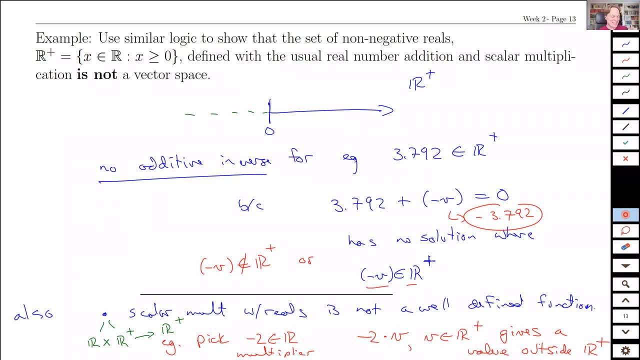 I think control theory. driving robotic cars is a much more interesting motivation to do linear algebra, But it's also the example of solving linear systems and how many solutions are there. is something we're going to return to inside this course, unlike control theory. 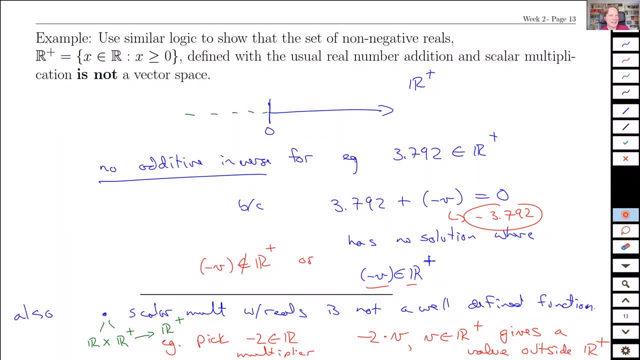 So it's meant to kind of set the stage for that. But I think you're going to figure it out just fine when we get to that, And I think it's like week six, seven. So, yeah, we're not going to finish the week one notes. 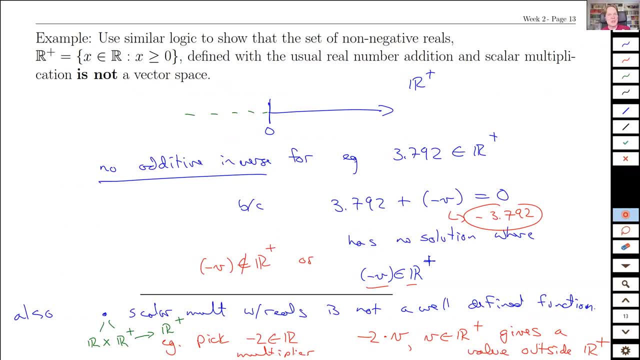 It's not the best use of our time. I think Grappling with vector spaces- which is new, I think- is where we're going to take some time. Yeah, So what's the difference between those two sets? Sorry, go ahead. 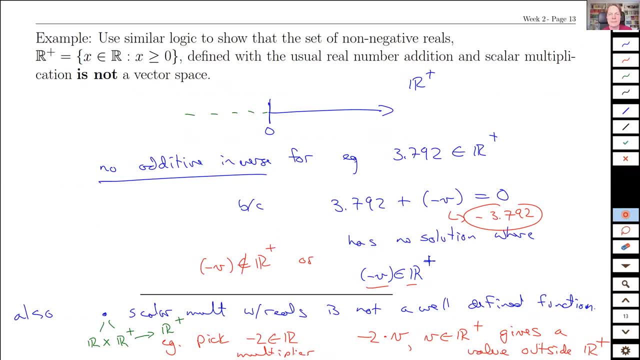 Yeah, sorry, Just a follow up question to Emma's question. So like we don't have to until we cover it in week six, seven, We won't really see any of that until we cover it later on. You've actually seen it. 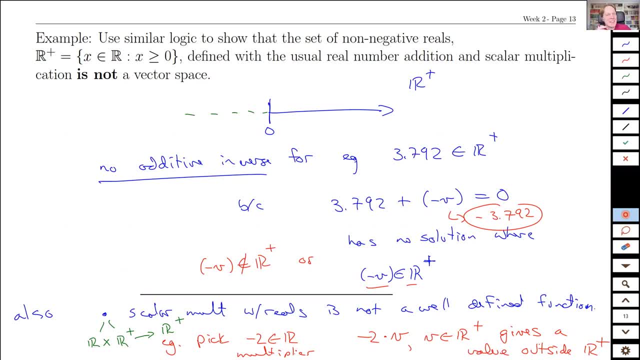 Like it's two equations, two unknowns. There's nothing new there. The only thing that's new is sort of the observation of: sometimes there's no answers, Sometimes there's a single answer And gosh, there's other things, Sometimes there's an infinite number of answers. 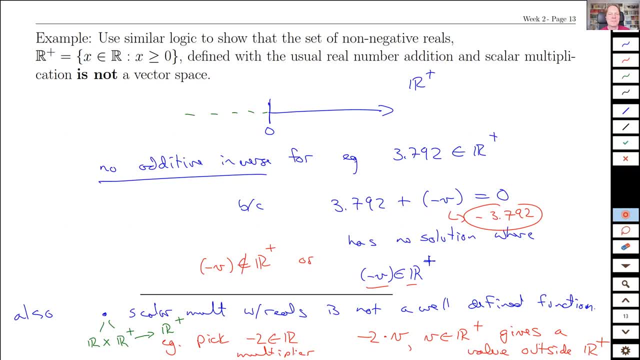 Is that a pattern? That's really. all we're doing is setting the seeds for that observation. Okay, perfect, Thank you. Okay, Thanks for checking. So the difference between R plus versus the natural numbers. So if I put them side by side here, the let me move this down a little bit. 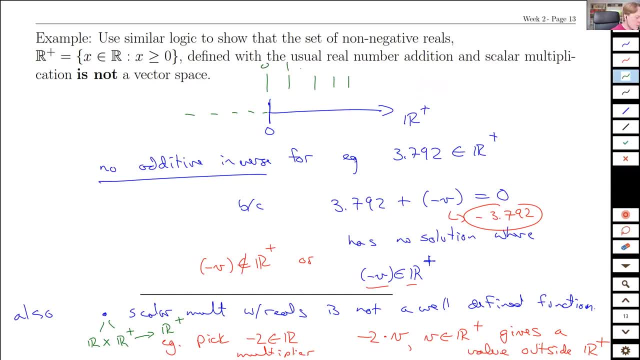 So R plus is this guy, And the natural numbers are just the integers that are zero or larger. So the real numbers Has all this stuff in between. So 1.793 is in the reals, 1.7393 is not in the natural numbers. 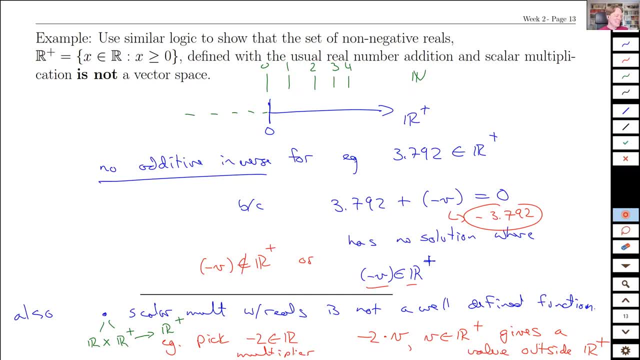 That's the difference. It's the again that continuity thing. All the space between the real numbers is filled in. It's not filled in for the naturals. There's all these gaps. I just have a question about the notation you used earlier for showing vector spaces. 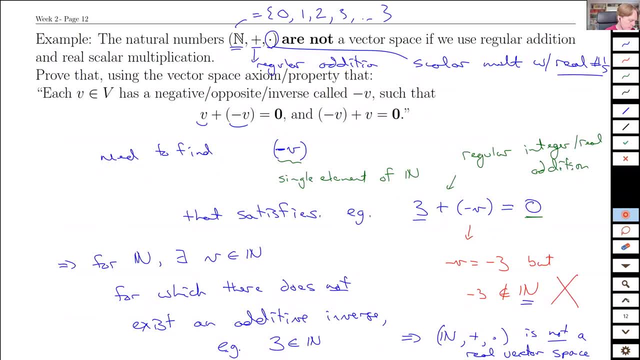 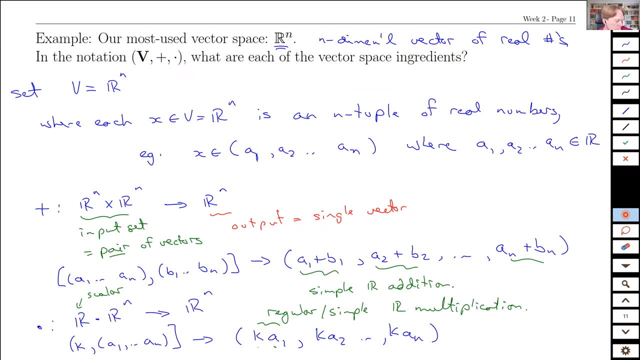 Okay, When you have something that's, you wrote it out. You said we're being specific. It's V And then comma plus like: yeah, just like that. Basically, what that means is that it's two sets of vectors that we can multiply and add. 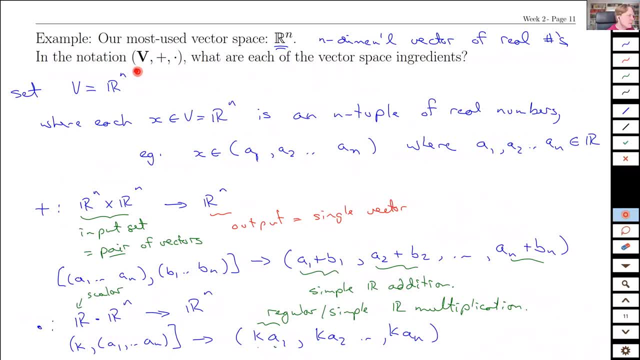 Not that we necessarily are doing them Yes and no. So again, it feels kind of silly with this kind of thing, Like when we use plus and scalar multipliers, What you'll often see- I think it's actually in the web work. 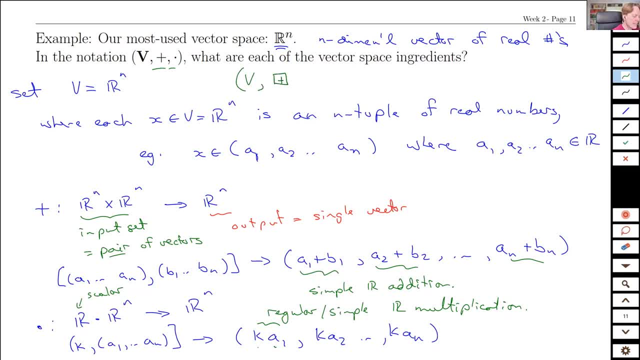 If we're going to do something weird, we might put a new symbol in here instead, And you know some cross with a circle in it, like that. That would be an indicator that you might know the set. Like maybe we would do this with the reals. 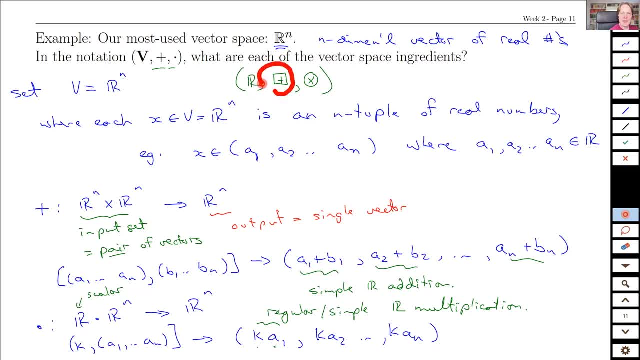 So you're gonna use the real numbers as your building blocks, But then you're going to have an addition operator that we're going to define for you. That's not the regular addition operator, And we'll typically try to pick a different symbol. 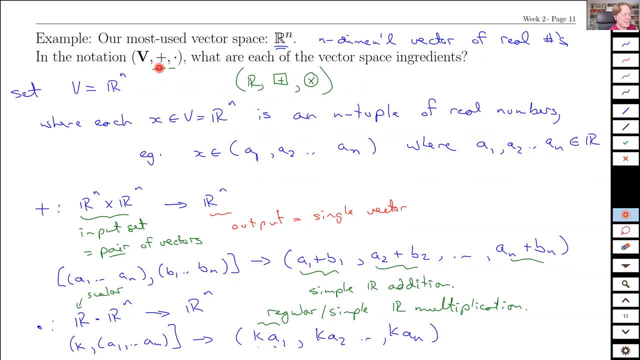 The idea is it's our set and then it's whatever we're going to call addition And then whatever we're going to call scalar multiplication, in that order. And if we're going to change things up And use weird rules for these things, 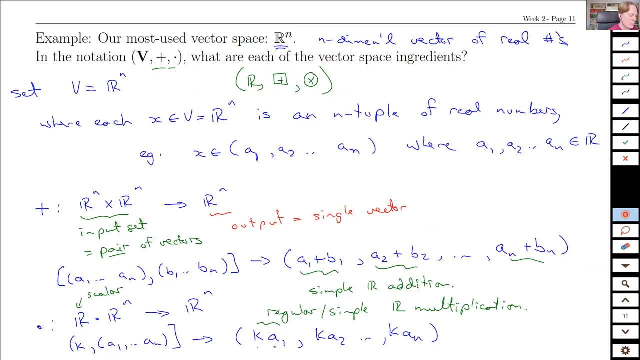 We'll make that explicit And then we'll define them. on the next line We'll say: by the way you know, this means if I take two real numbers, I'm going to get the sum of them plus five or something weird.